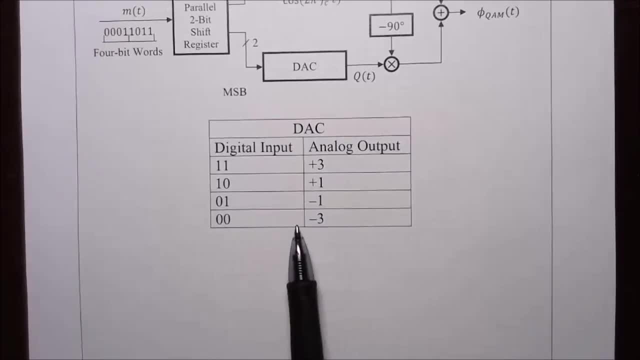 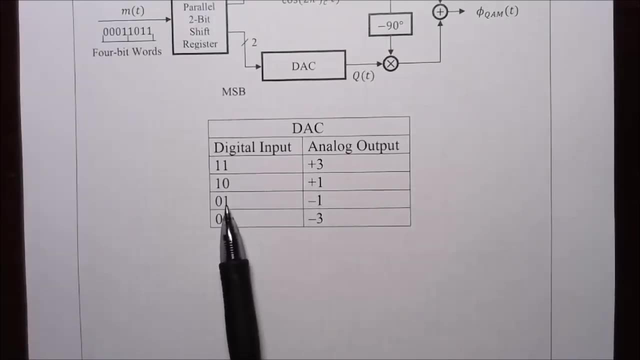 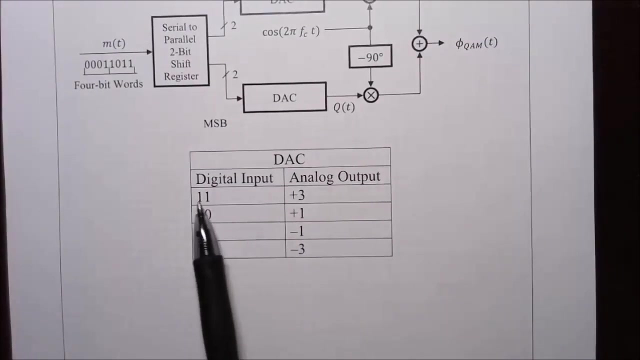 This digital-to-analog converter produces an output of minus 3 volts. so 0-0 input maps to minus 3 volts out. 0-1 input maps to minus 1 volt out. 1-0-n is plus 1 volts out and 1-1-n maps to 3 volts out. 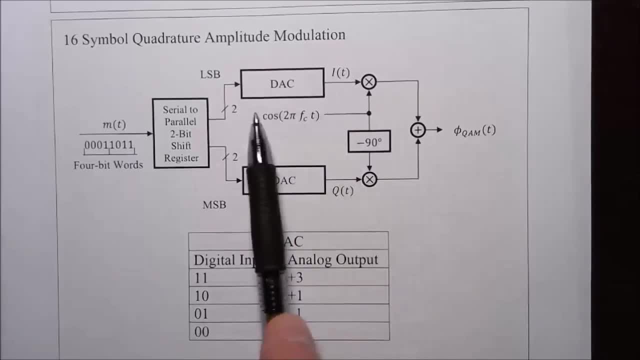 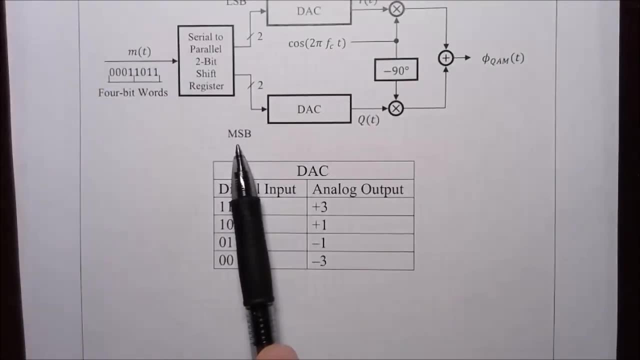 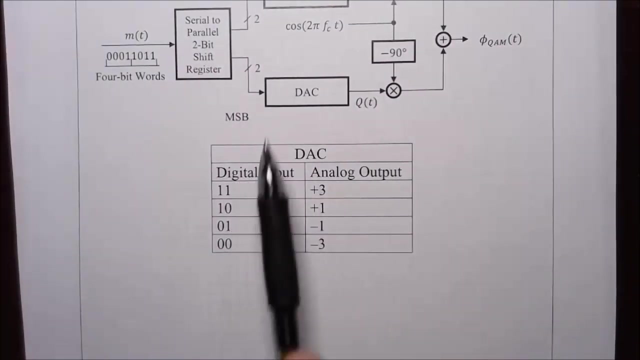 That is, the in-phase signal which is mixed with the in-phase carrier and then applied to the summing amplifier. The two most the more significant bits go through the quadrature mixer. Using the same digital-to-analog converter with two bits, there's four possible inputs. 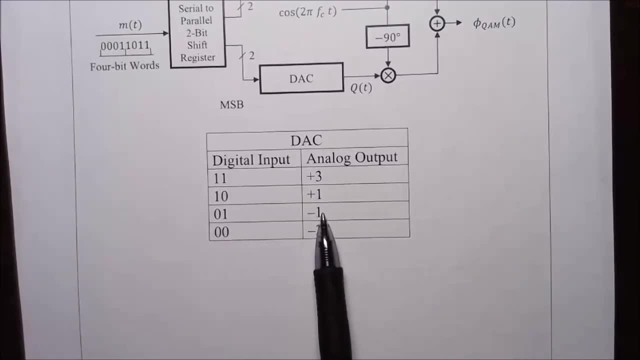 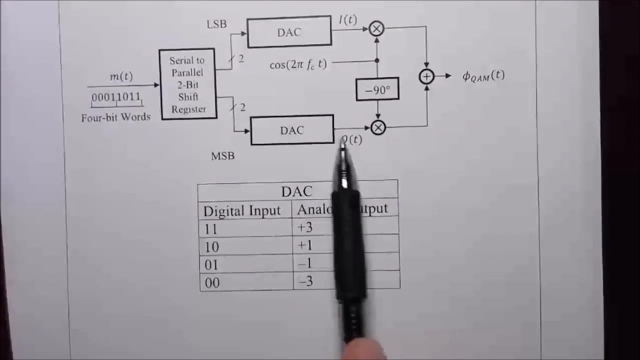 0-0,, which maps to minus 3.. 0-1 maps to minus 1.. 1-0 maps to plus 1, and 1-1 maps to plus 3.. And then that is the quadrature signal. 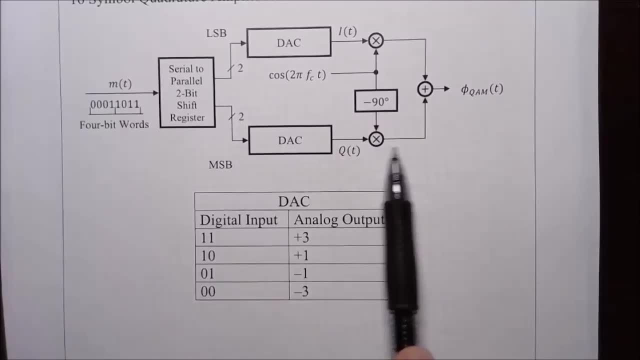 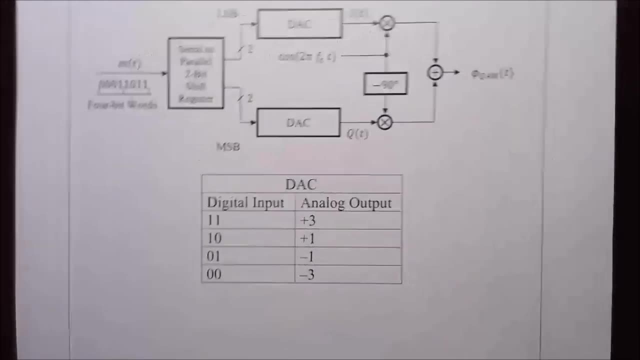 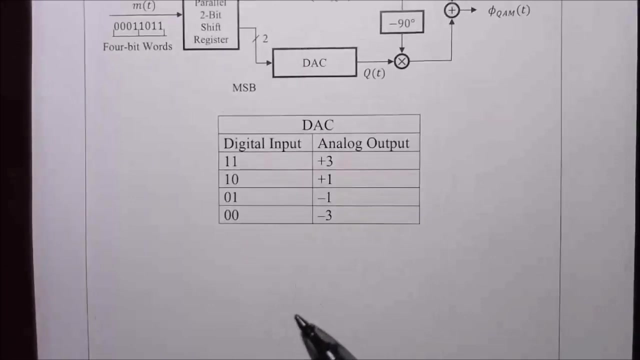 which is then mixed with the quadrature carrier and added to form a quadrature amplitude modulated signal, And the amplitude will be clearly modulated In this signal. it wasn't with the other phase, shift keyed signals. So what I want to do, I want to draw the constellation diagram. 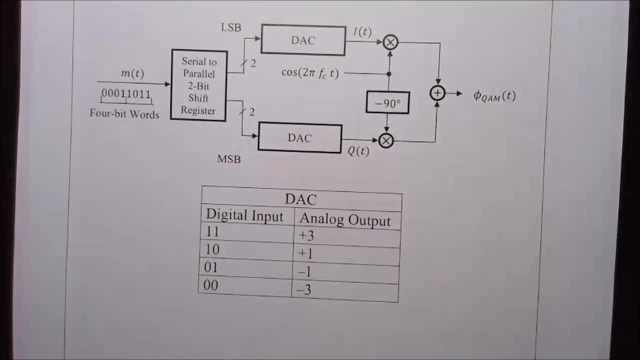 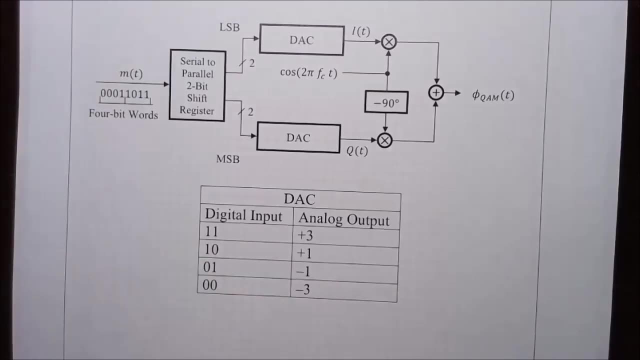 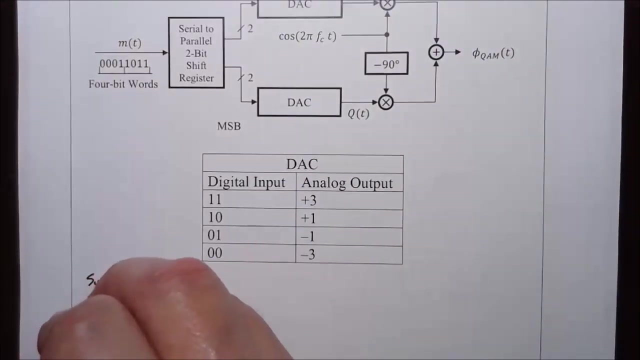 This is what it says right there. Draw the constellation diagram, So we've got four-bit words. With four bits there's 16 possible combinations for the signal. So I'll start. We'll start with 0-0,. 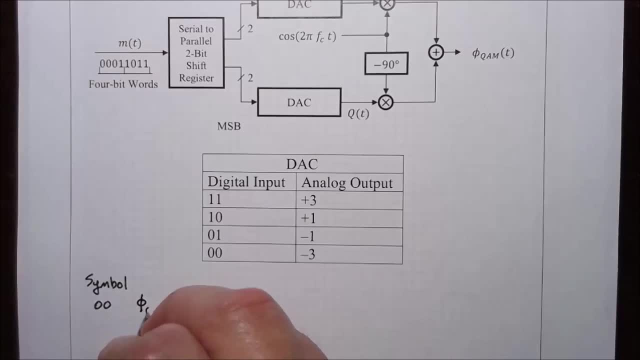 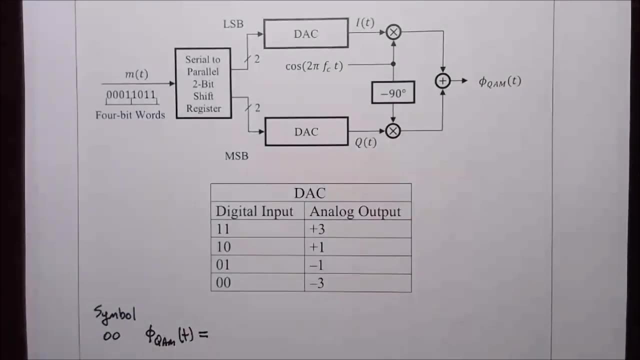 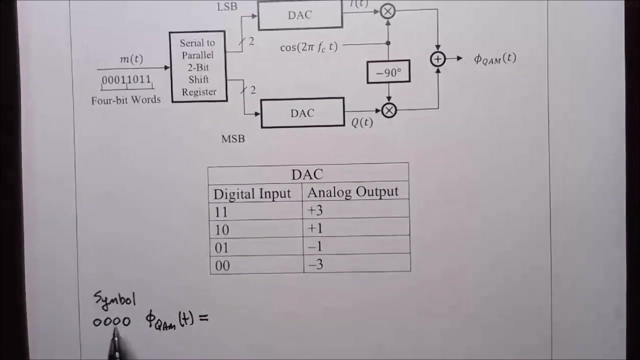 and we will find the quadrature AM signal as a function of time. So I'm sorry, the symbol is not 0-0, but 0-0-0-0.. We're using four bits. Two bits for the more significant bits. 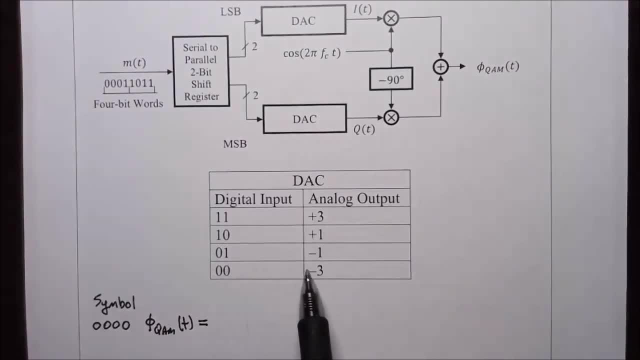 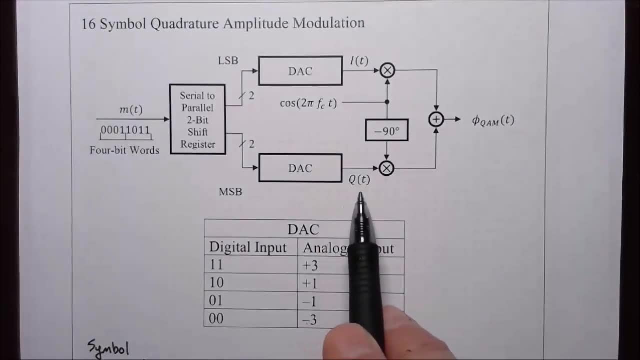 two bits for the least significant bits. Both of these map to minus 3.. So the in-phase signal is minus 3, and the quadrature signal is minus 3.. So we have, for the in-phase carrier, minus 3 times cosine. 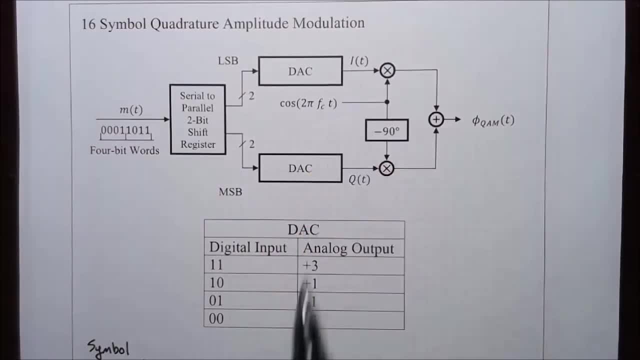 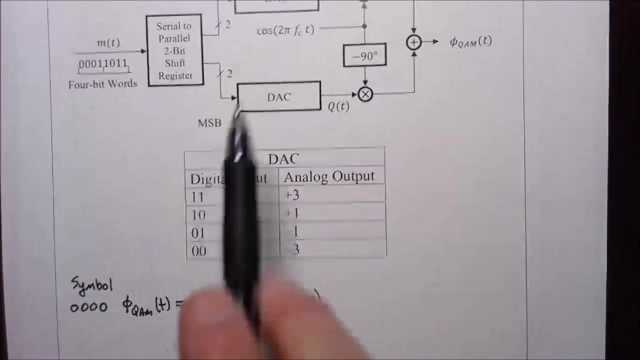 So let me put the minus into a phase shift and call this 3 times cosine 2, pi, fct minus 180 degrees. Okay, so, I'm sorry, there we go. This is minus. so the least significant bit, 0-0, maps to minus 3.. 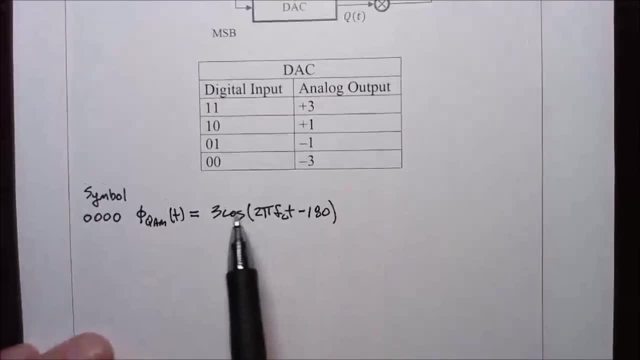 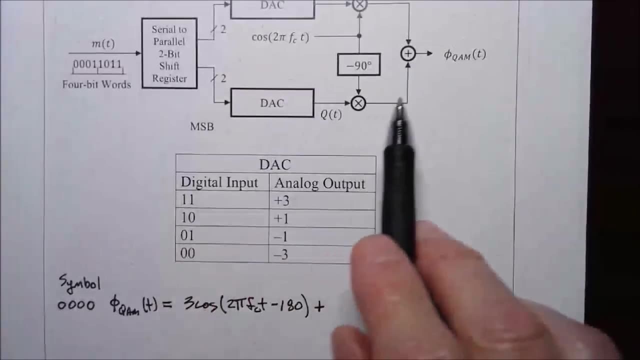 So we have minus 3 times cosine. So I'll put the minus sign into the phase angle: 3 cosine 2 pi fct, and we're adding to that the signal through the bottom. That's the more significant bit. 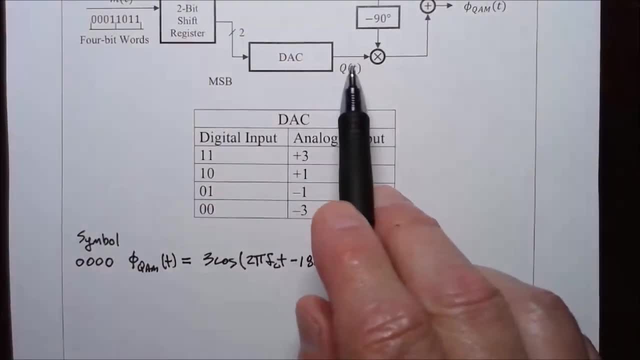 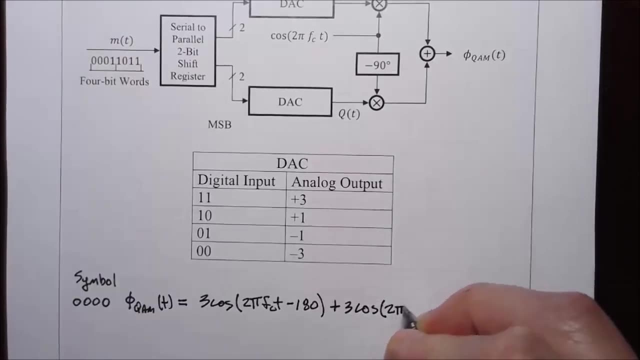 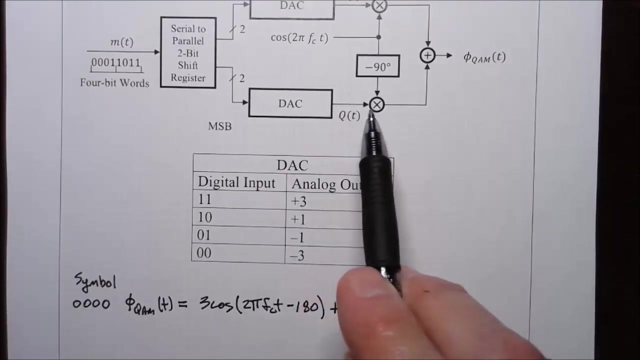 Again 0-0. maps to minus 3.. So this is minus 3 times the quadrature carrier 2 pi fct. And now let's put the minus sign into the phase angle, So we've got a minus 180 and a minus 90.. 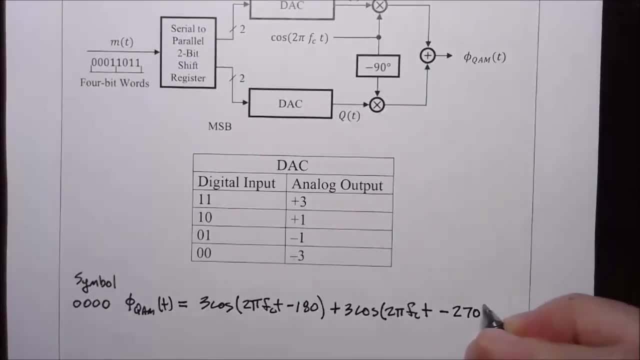 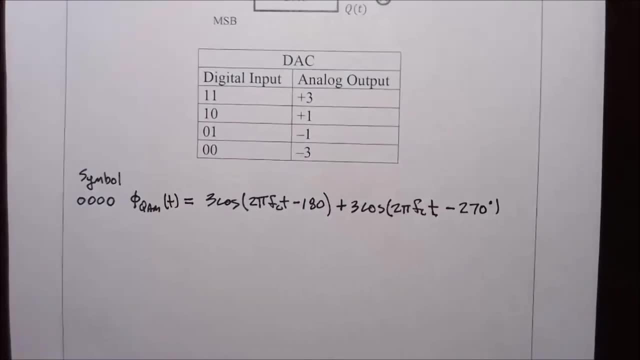 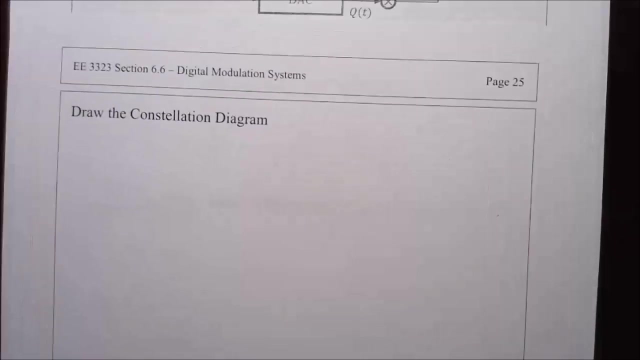 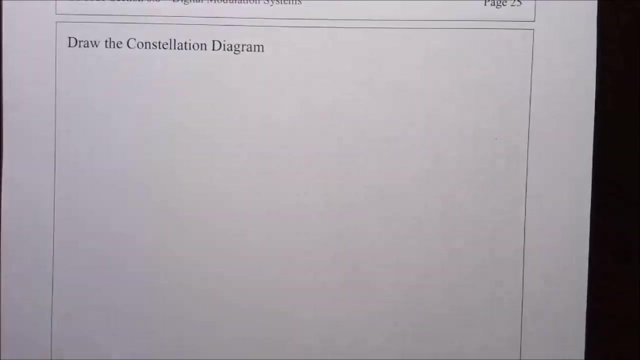 So the total is minus 270 degrees. Okay, so this is the signal that we are going to draw to map onto the constellation diagram. So let me start with the, with the real axis and the imaginary axis, And let's see if I can keep this. 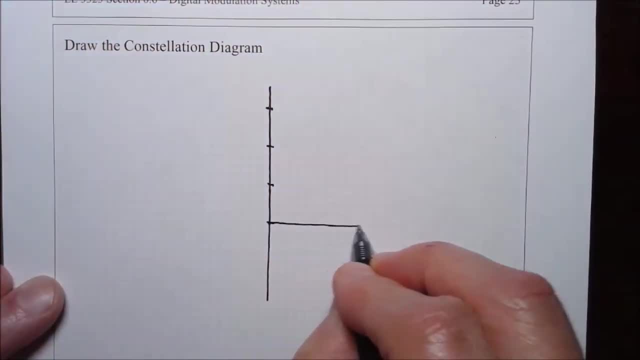 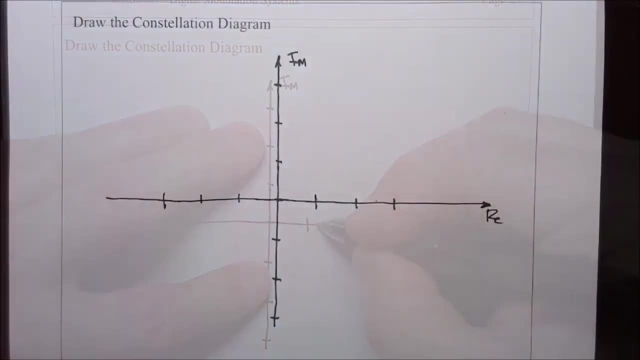 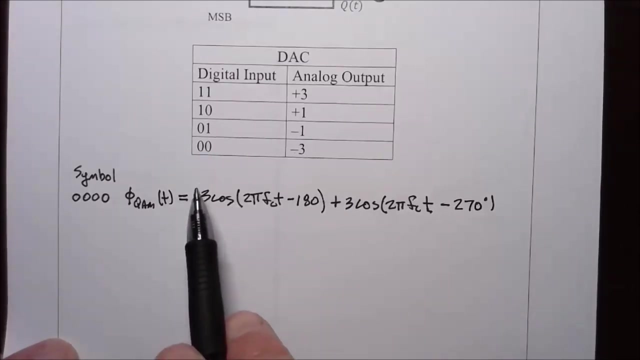 Okay, this, let's put the real axis here. This is the imaginary axis And I'm putting in some tick marks. So we want to plot the phasors for these two sinusoids. The first has an amplitude of 3 and an angle of minus 180 degrees. 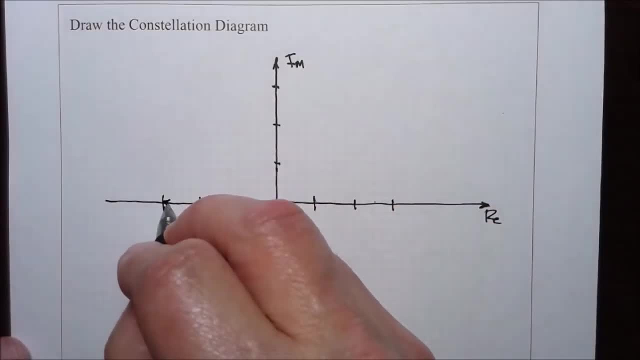 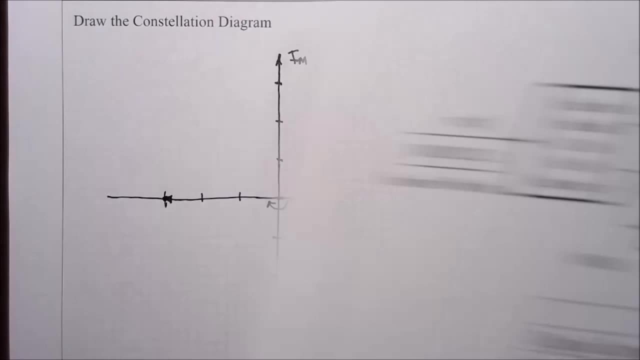 So that's an amplitude of 1,, 2, 3.. So the arrow points to here And the angle is minus 180.. That's to this point. The next has an amplitude of 3 and an angle of minus 270 degrees. 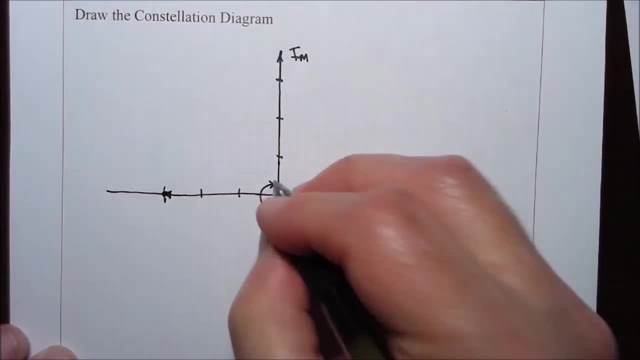 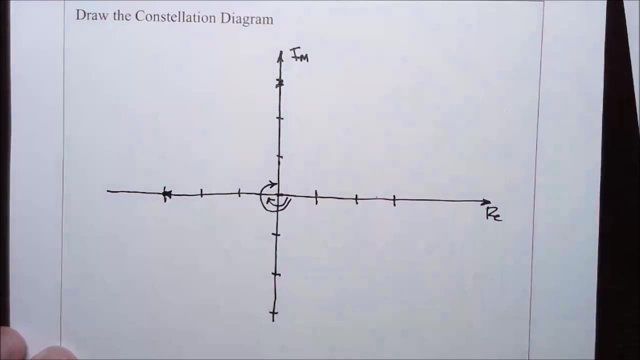 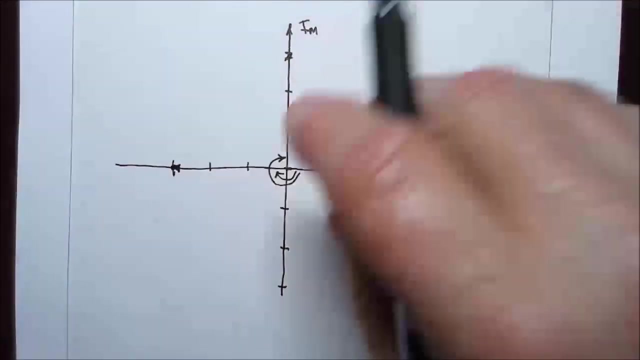 So minus 270 degrees and a magnitude of 1,, 2,, 3.. And this takes is a vector that points to that point. When we add the two vectors together, we get a point that falls, If I can hit it right there: 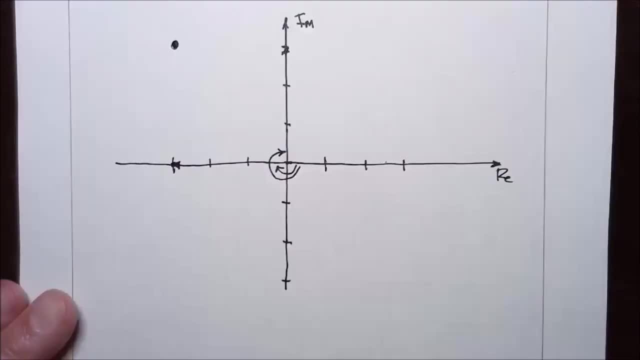 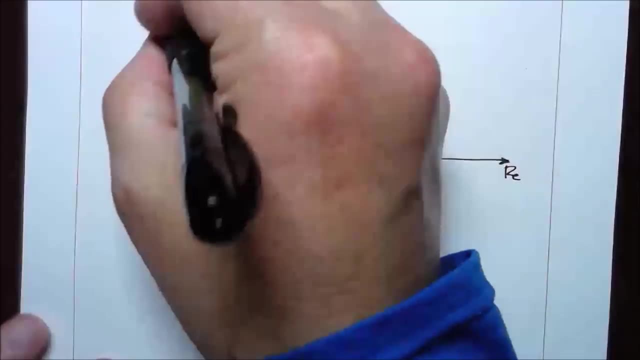 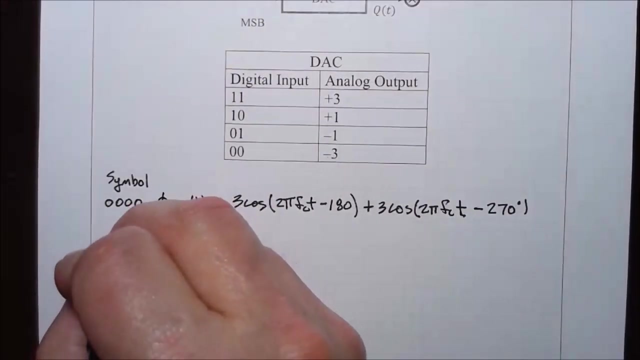 This is the point in the constellation diagram that corresponds to the symbol 0000.. So this is for 0000.. Okay, let's go to the next, Which is 0000.. 0000.. The square root of AM. 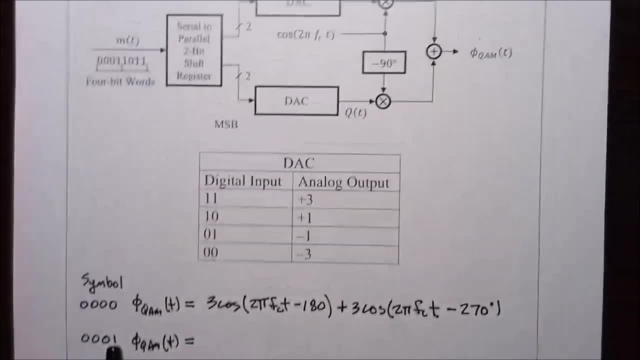 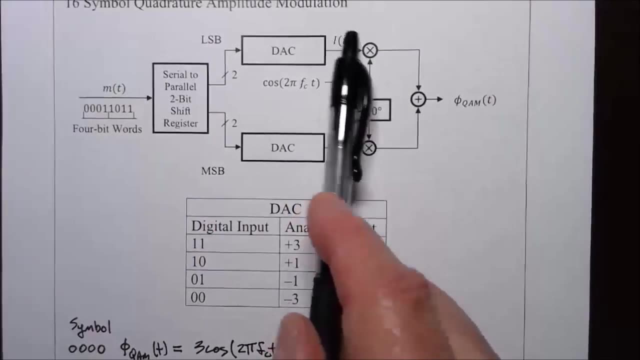 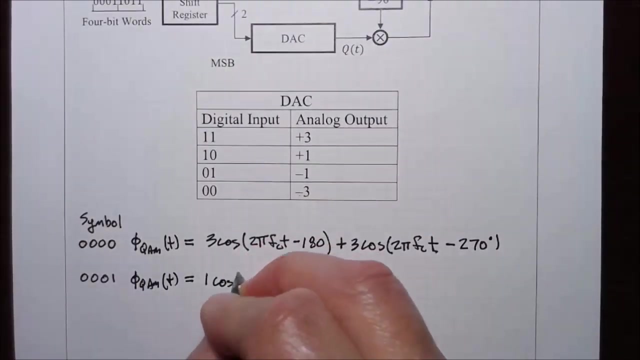 is now the least significant bit Are 01.. And 01 maps to minus 1.. So that's going to make the value of the in-phase signal minus 1.. Times this cosine, So that's going to be 1, times the cosine of 2pi FCT. 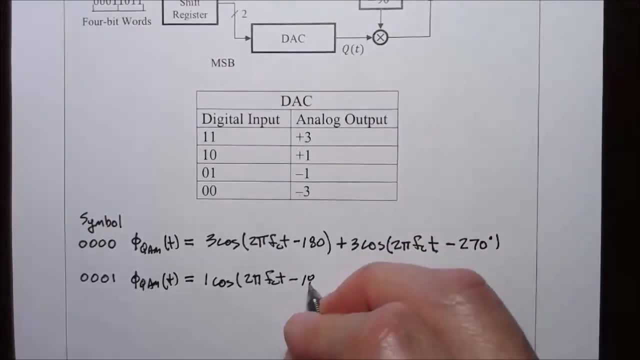 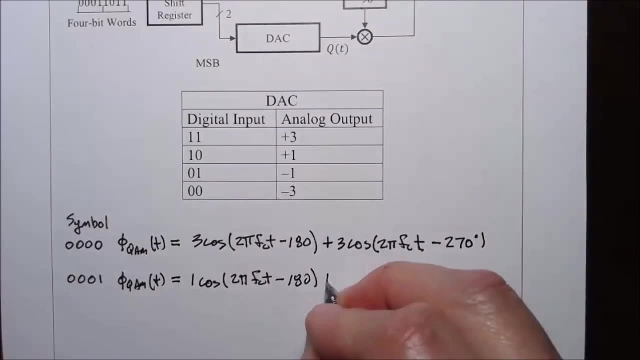 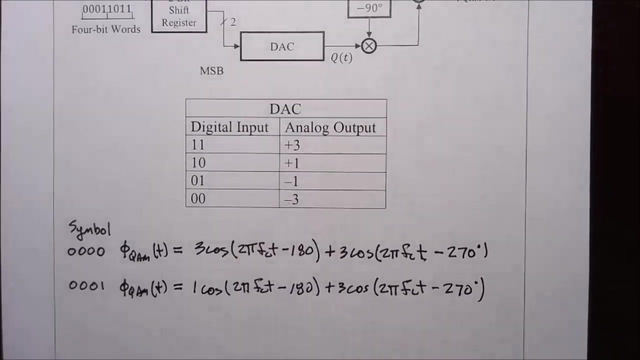 And I'll put the minus sign into the phase shift. and then zero, zero maps to exactly this same signal, again plus three, cosine two, pi, fct, minus 270 degrees. and now we plot the phasors. we have one with an angle of minus 180. 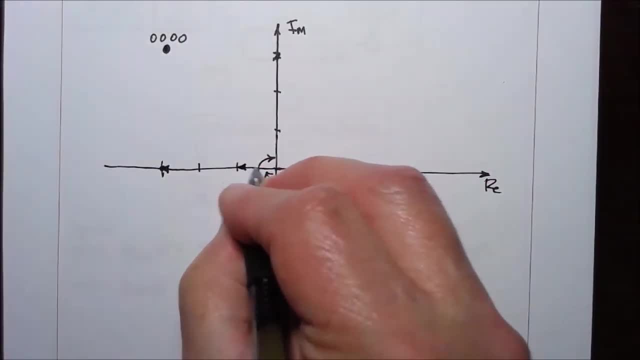 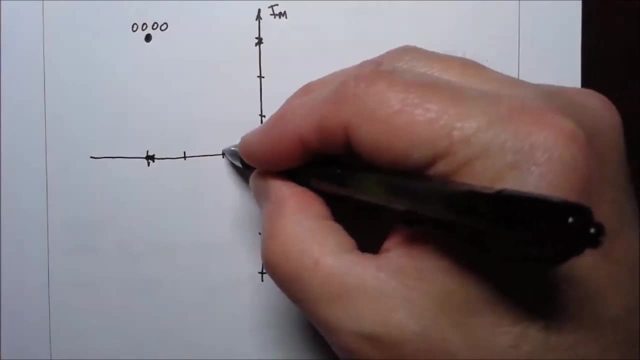 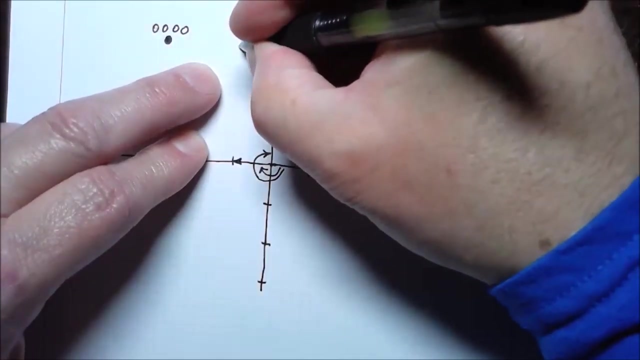 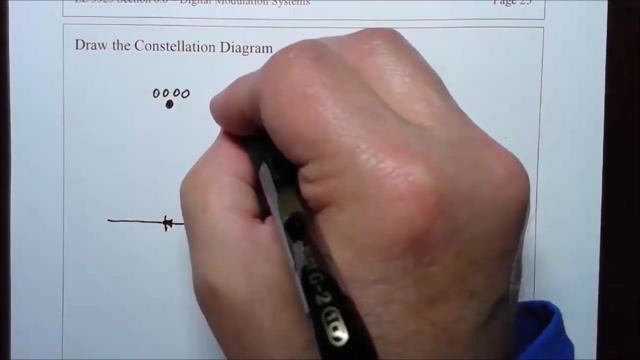 that points to this line. this is one with an angle minus 180 plus three with an angle of minus 270. so plus three with an angle of minus 270 gets us to. it looks like this point right there. so this point in the constellation diagram is for zero, zero, zero one. 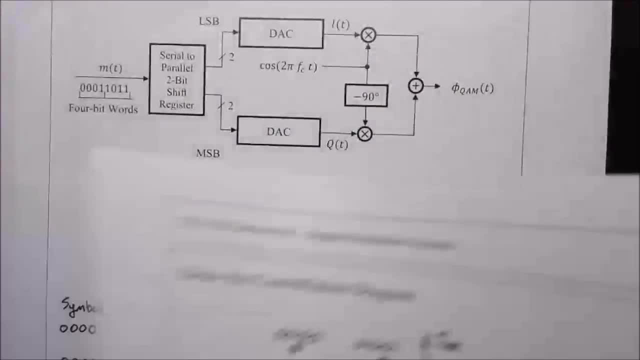 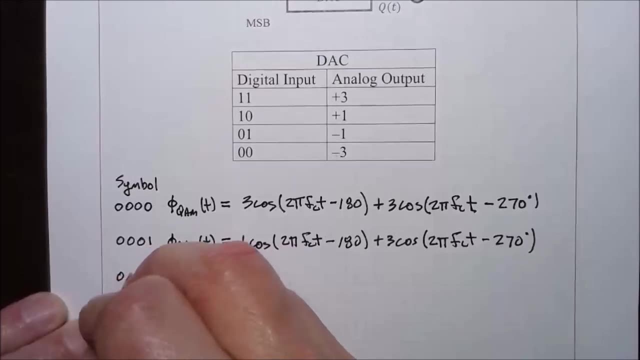 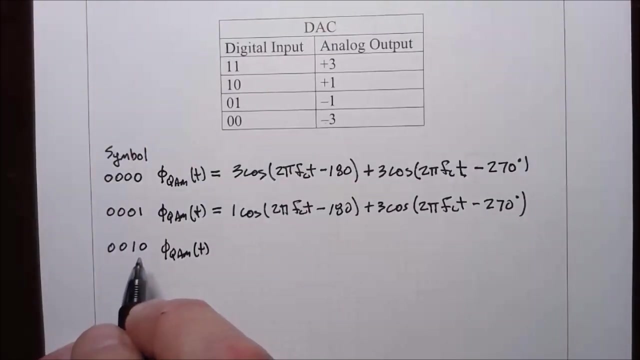 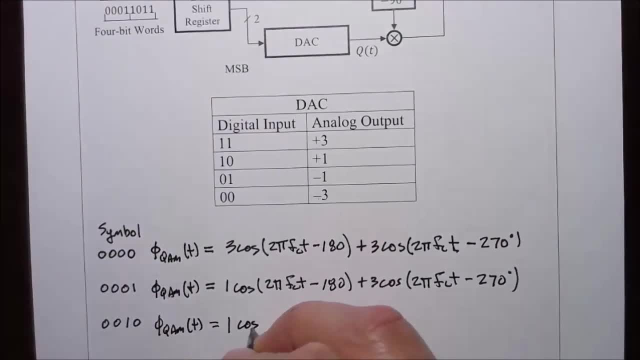 corresponds to plus one. so that's going to be one cosine two pi fct, and that's going to be one cosine two pi fct, and that's going to be one cosine two pi fct, and that's going to be one cosine two pi fct, minus zero degrees, because we're 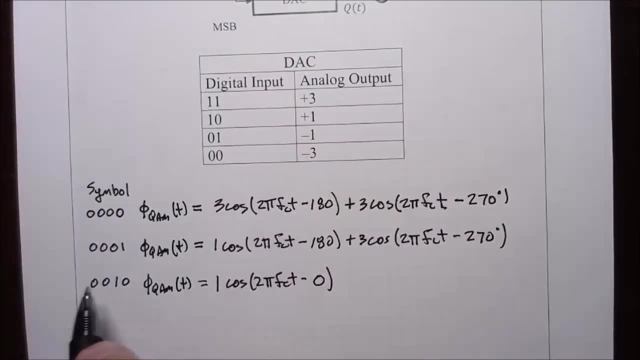 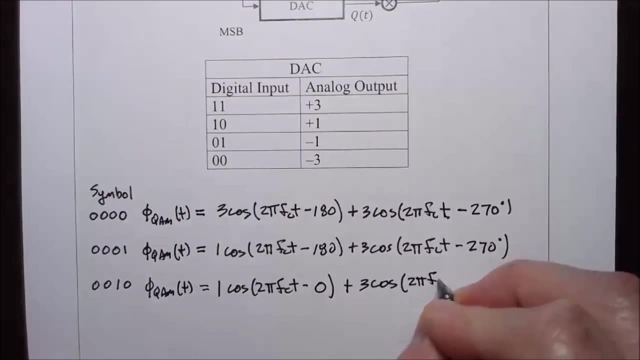 minus zero degrees. because we're minus zero degrees, because we're multiplying by plus one, and then for the multiplying by plus one, and then for the multiplying by plus one, and then for the more significant bit: zero, zero. we get more significant bit: zero, zero. we get more significant bit: zero, zero. we get the same plus three, cosine two, pi, fct. 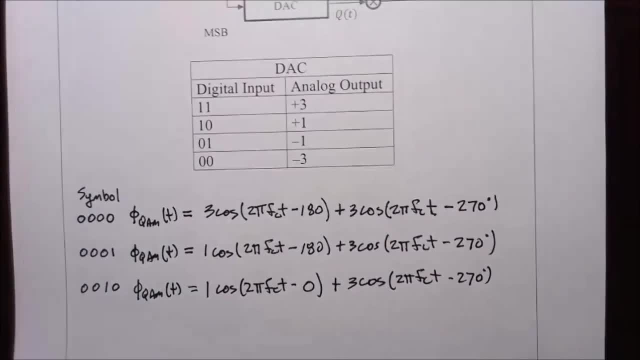 the same plus three cosine two pi fct. the same plus three cosine two pi fct minus 270 degrees. and we draw the we minus 270 degrees, and we draw the we minus 270 degrees, and we draw the. we draw the phaser we have, that's alright we. 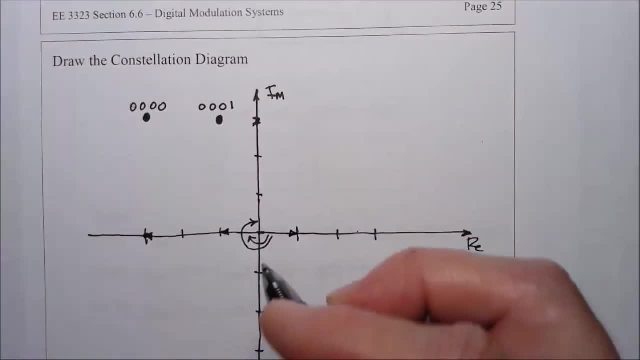 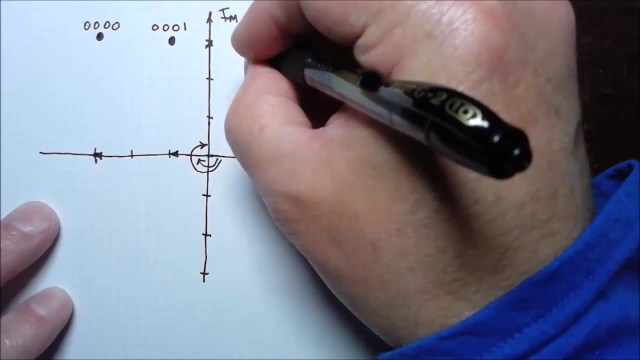 draw the phaser we have. that's alright. we draw the phaser we have, that's alright. we have one with an angle of zero plus. have one with an angle of zero plus. have one with an angle of zero plus three, three, three with an angle of minus 270. there for. 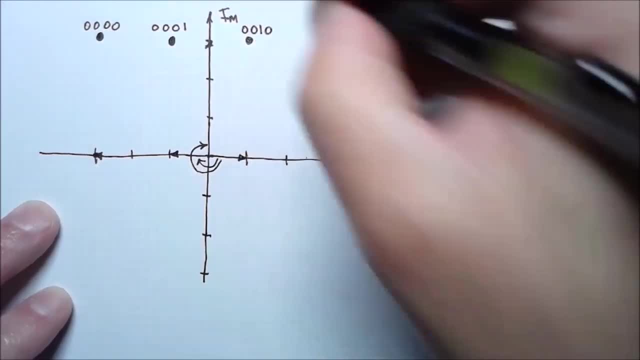 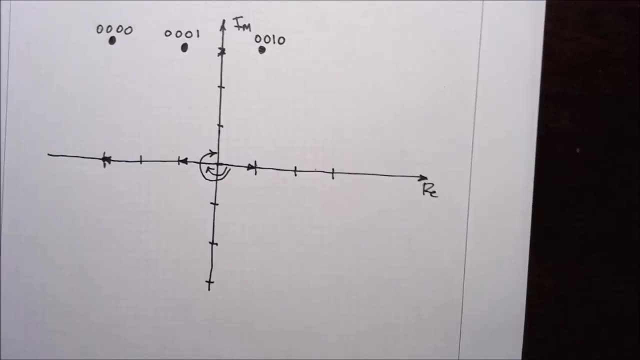 with an angle of minus 270 there for with an angle of minus 270 there for zero, zero, one, zero. and I'm willing to zero, zero, one, zero, and I'm willing to zero, zero, one, zero and I'm willing to bet zero, zero, one one falls right here. 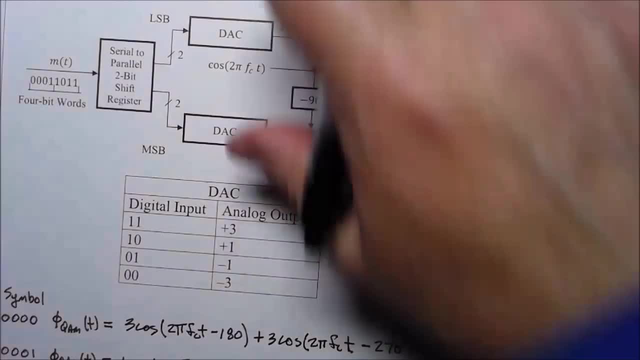 bet zero, zero one one falls right here. bet zero, zero one one falls right here. but let's let's zero zero one one fee. but let's let's zero zero one one fee. but let's let's zero zero one one fee. Q am the two least significant bits. 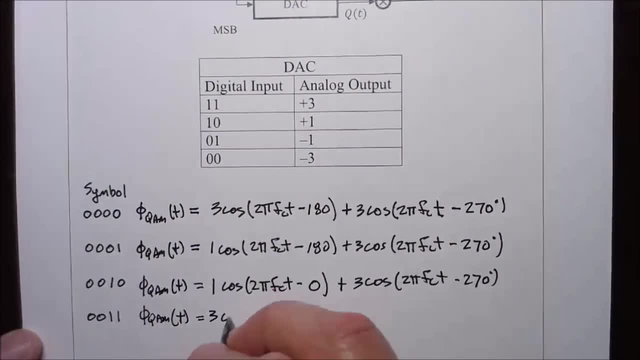 Q am the two least significant bits. Q am the two least significant bits, mapped plus three. so that's going to be mapped plus three, so that's going to be mapped plus three, so that's going to be three times cosine 2, PI, FCT minus zero. 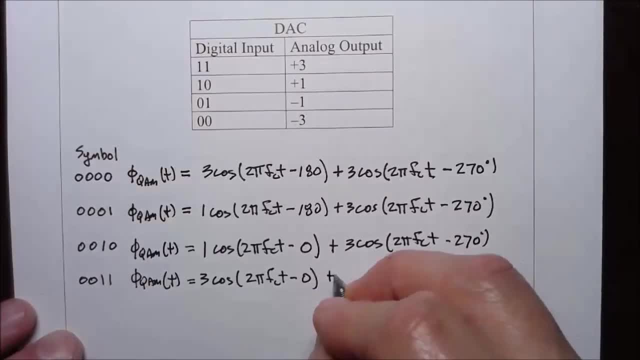 three times cosine 2 PI FCT, minus zero. three times cosine 2 PI FCT- minus zero. because it's got a plus sign, and then because it's got a plus sign, and then because it's got a plus sign, and then for zero, zero, we get the same three. 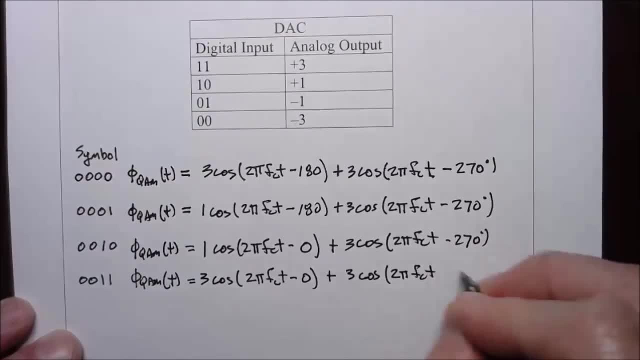 for zero zero. we get the same. three for zero zero. we get the same three times the cosine 2 PI FCT minus 270 times the cosine 2 PI FCT minus 270 times the cosine 2 PI FCT minus 270 degrees. so an angle of magnitude 3 at an. 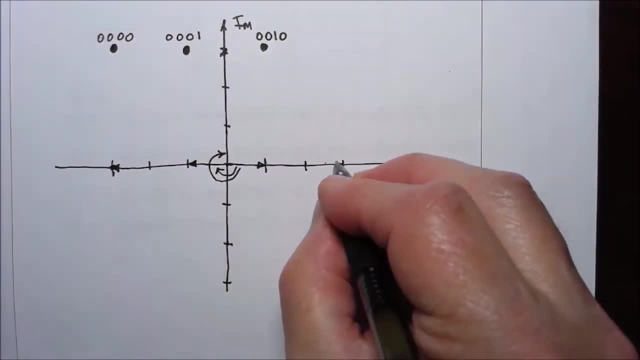 degrees, so an angle of magnitude 3 at an degrees, so an angle of magnitude 3 at an angle of zero. points out to this angle of zero, points out to this angle of zero, points out to this direction. magnitude 3: angle 0 plus 3 at. 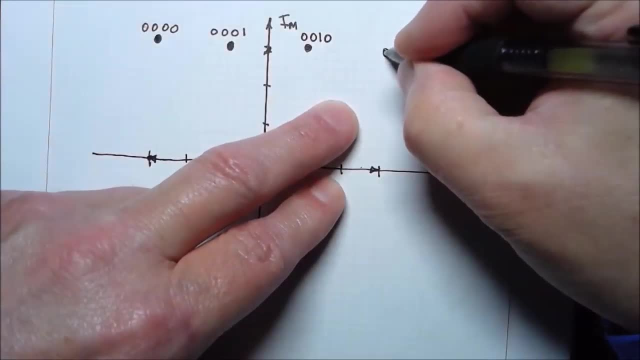 direction: magnitude 3, angle 0 plus 3. at direction: magnitude 3, angle 0 plus 3, at an angle of 70, and right there, this is an angle of 70, and right there, this is an angle of 70, and right there, this is four zero, zero, one one. so those are the. 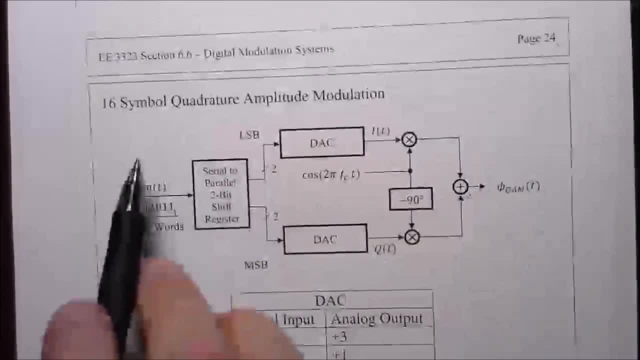 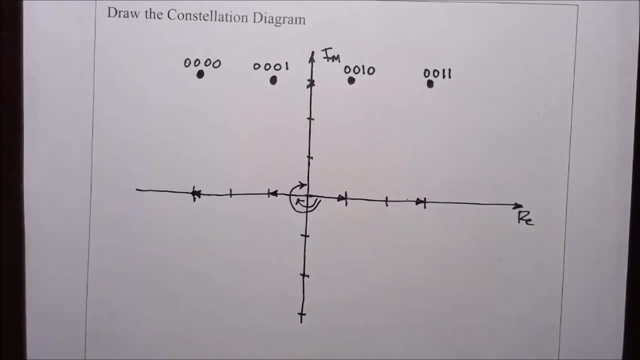 four zero zero one one. so those are the four zero zero one one. so those are the first four points in a 16 symbol, first four points in a 16 symbol, first four points in a 16 symbol. quadrature a in signal. let me stop the. 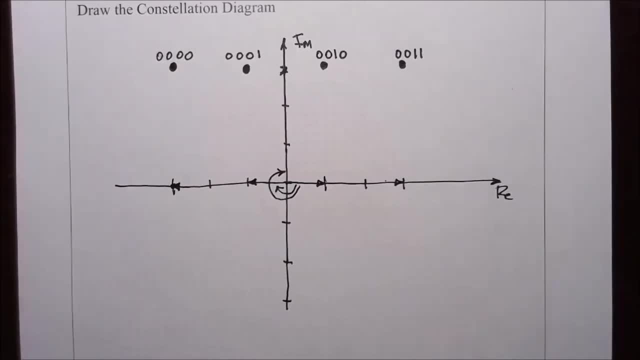 quadrature a in signal. let me stop the quadrature a in signal. let me stop the recording and I will think about where recording and I will think about where recording and I will think about where the rest of them fall completed: the. the rest of them fall completed: the. 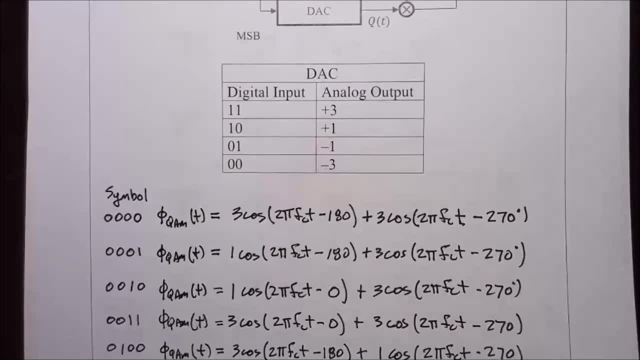 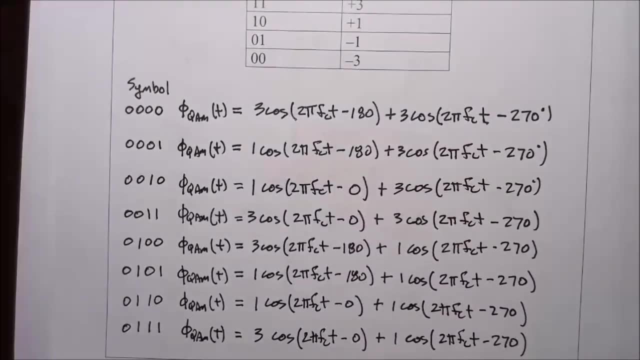 the rest of them fall. completed the equations for all 16 of the symbol equations for all 16 of the symbol equations for all 16 of the symbol symbols in this 16 symbol quadrature AM symbols in this 16 symbol quadrature AM symbols in this 16 symbol quadrature AM system, and there's symbols 0, 1, 2, 4, 5, 6, 7. 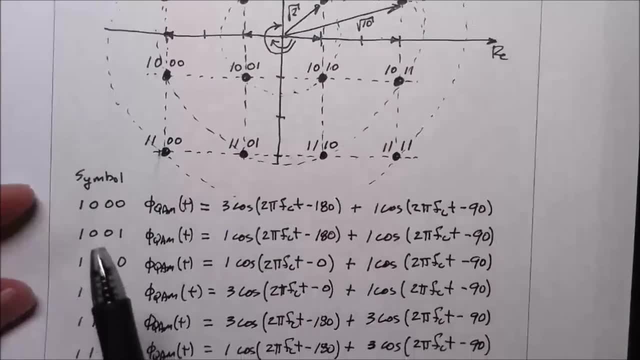 system and there's symbols 0, 1, 2, 4, 5, 6, 7. system and there's symbols 0, 1, 2, 4, 5, 6, 7 and here symbols 8, 9, 10, 11, 12, 13, 14 and. 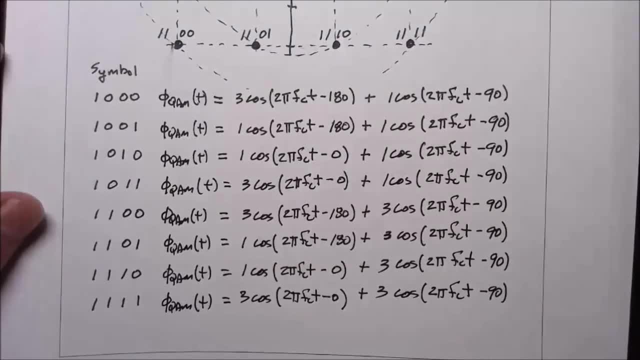 and here symbols 8, 9, 10, 11, 12, 13, 14, and, and here symbols 8, 9, 10, 11, 12, 13, 14 and 15, and you can look through them at 15 and you can look through them at: 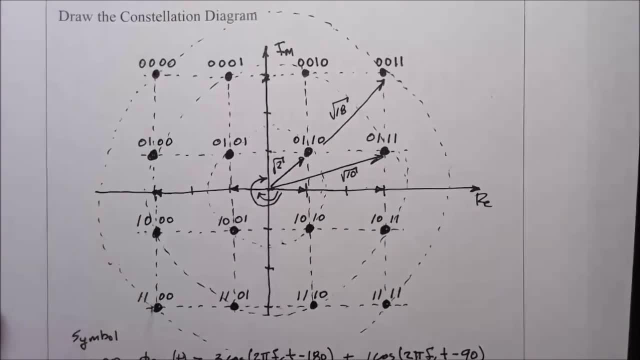 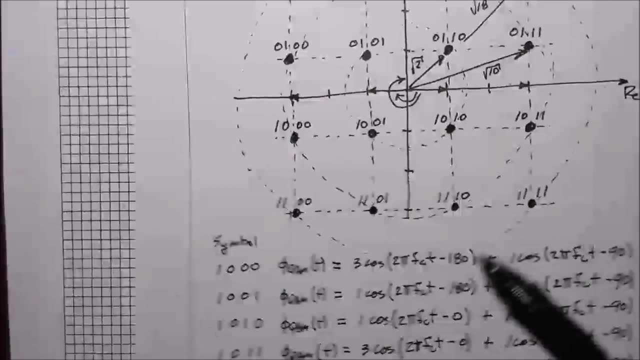 15, and you can look through them at your convenience. and this is the the 16 your convenience. and this is the the 16 your convenience. and this is the the 16 symbol constellation diagram with with symbol constellation diagram with. with symbol constellation diagram with with all 16 of the symbols at an individual. 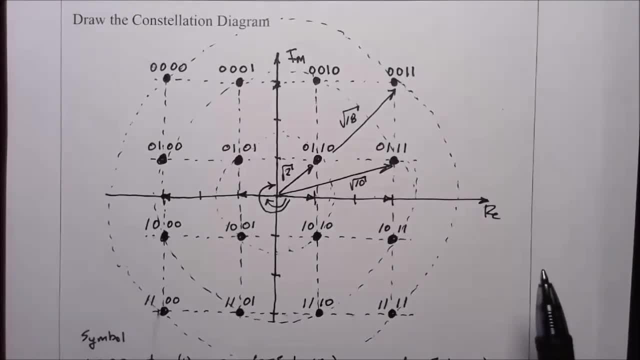 all 16 of the symbols at an individual, all 16 of the symbols at an individual point in the constellation diagram. this point in the constellation diagram, this point in the constellation diagram, this is a clearly different amplitudes for is a clearly different amplitudes for. 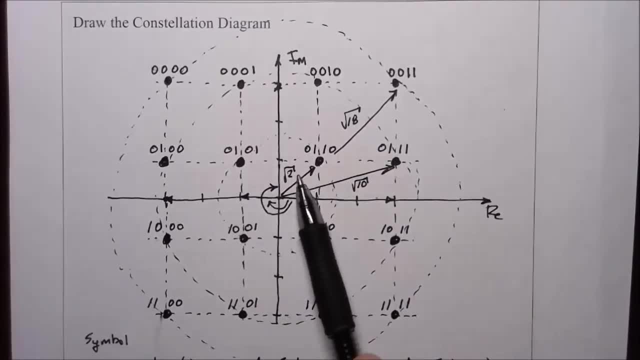 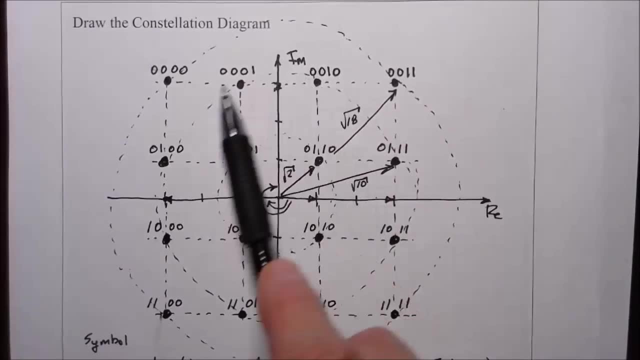 is a clearly different amplitudes for different symbols. these four symbols in different symbols. these four symbols in different symbols. these four symbols in the middle have an amplitude of square. the middle have an amplitude of square. the middle have an amplitude of square root. 2, 1, 2, 3, 4, 5, 6, 7, 8 symbols have root. 2, 1, 2, 3, 4, 5, 6, 7, 8 symbols have root: 2, 1, 2, 3, 4, 5, 6, 7, 8 symbols have an amplitude of square root of 10 and then. 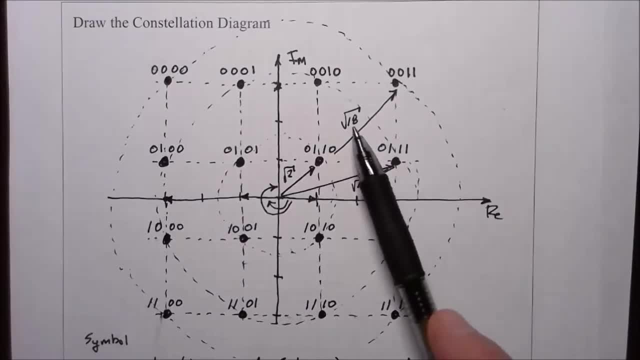 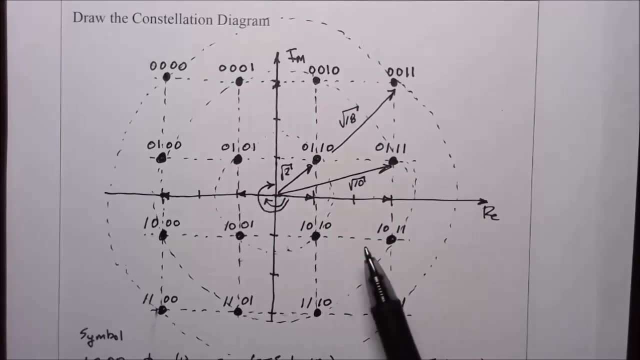 an amplitude of square root of 10, and then an amplitude of square root of 10, and then 1, 2, 3, 4 symbols have a amplitude of the 1, 2, 3, 4 symbols have a amplitude of the 1, 2, 3, 4 symbols have a amplitude of the square root of 18. now, this is just just. 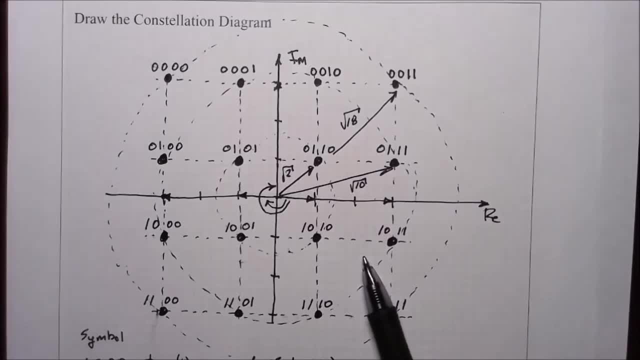 square root of 18. now, this is just just square root of 18. now, this is just just one way of of making a 16 symbol. one way of of making a 16 symbol, one way of of making a 16 symbol, quadrature, am system and the 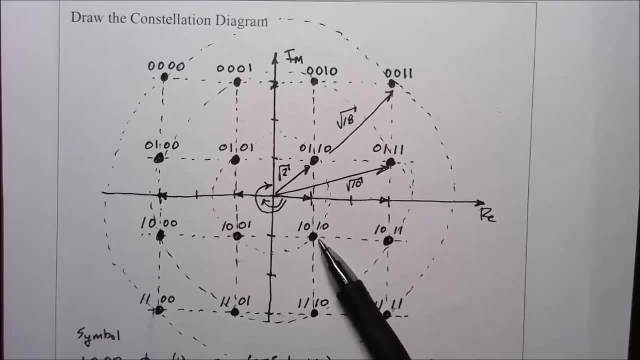 quadrature am system and the quadrature am system and the constellation diagram for it, these, these constellation diagram for it, these, these constellation diagram for it, these, these points can be placed. points can be placed. points can be placed in a number of places, depending upon the the. 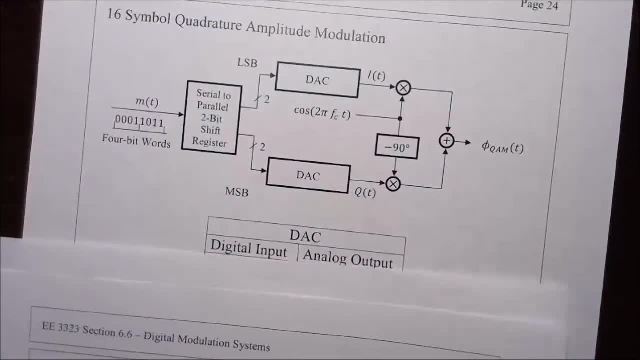 in a number of places, depending upon the, the in a number of places, depending upon the, the particulars of the of the system, particulars of the of the system, particulars of the of the system, and who's to say, without more analysis, and who's to say without more analysis. 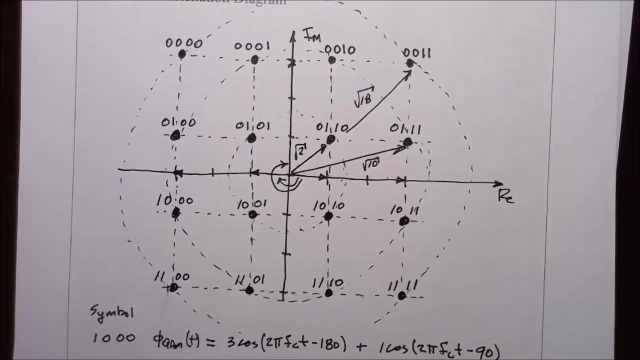 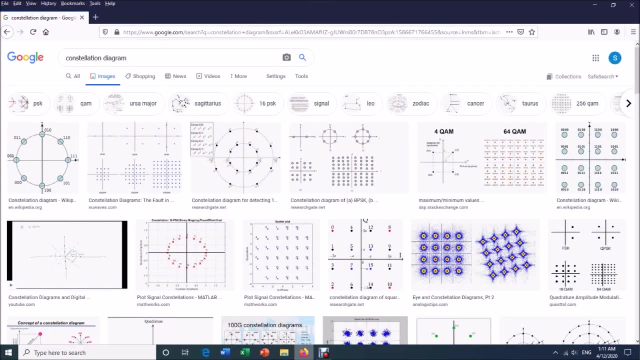 and who's to say, without more analysis, which which constellation diagram is? is which which constellation diagram is? is which which constellation diagram is? is more appropriate if you google more appropriate if you google more appropriate if you google constellation diagram on your computer. constellation diagram on your computer. 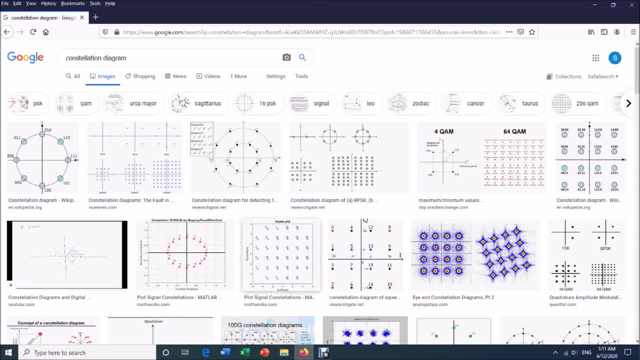 constellation diagram on your computer. this is the page that will come up, and this is the page that will come up, and this is the page that will come up and it shows several examples of how. it shows several examples of how. it shows several examples of how constellation diagrams may be designed. 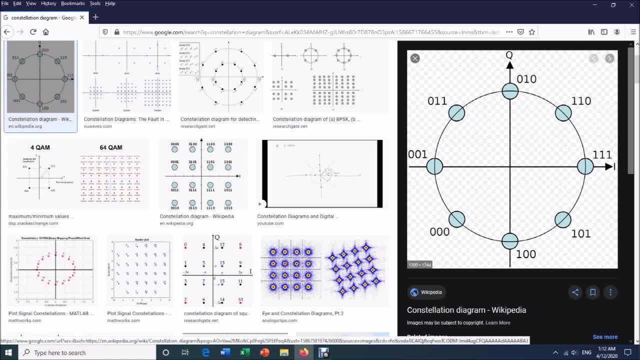 constellation diagrams may be designed. constellation diagrams may be designed. this is a 3-bit constellation diagram. this is a 3-bit constellation diagram. this is a 3-bit constellation diagram with 1, 2, 3, 4, 5, 6, 7, 8 symbols. 0 0 0. 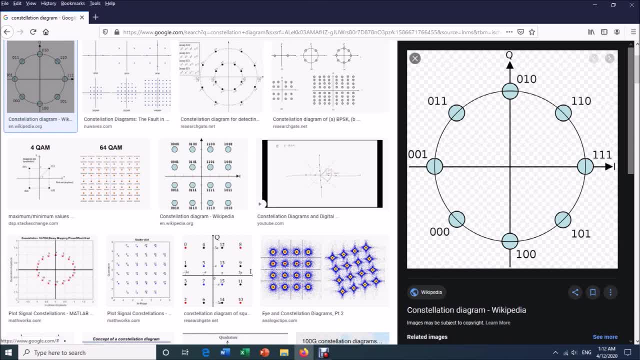 with 1, 2, 3, 4, 5, 6, 7, 8 symbols 0 0, 0. with 1, 2, 3, 4, 5, 6, 7, 8 symbols 0 0, 0 through 1 1, 1. that's one way of doing it. 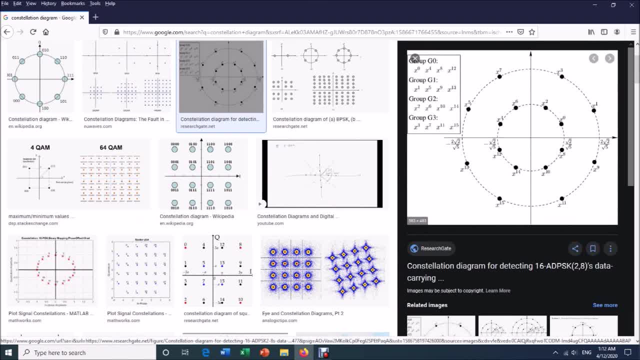 through 1 1 1. that's one way of doing it through 1 1 1. that's one way of doing it. here is a different way of doing a 16. here is a different way of doing a 16. here is a different way of doing a 16. symbol constellation diagram with. 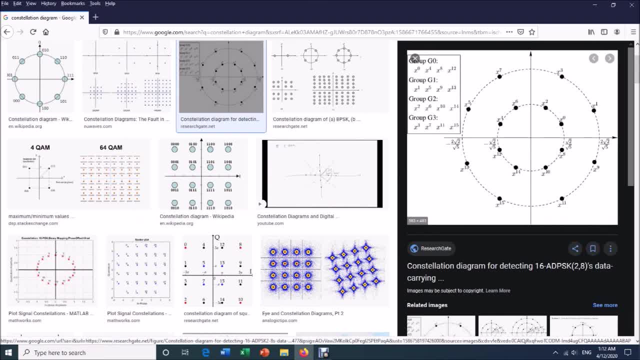 symbol constellation diagram with symbol constellation diagram with different locations and matt amplitudes, different locations and matt amplitudes, different locations and matt amplitudes, and phase angles and phase angles and phase angles. for the symbols: now one of some of. for the symbols, now one of some of. 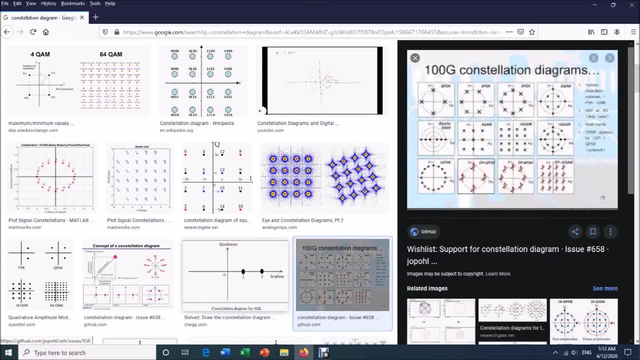 for the symbols. now, one of some of these designs may be preferred over other. these designs may be preferred over other. these designs may be preferred over other designs, depending upon other designs. depending upon other designs, depending upon other circumstances in designing the system. so circumstances in designing the system. so. 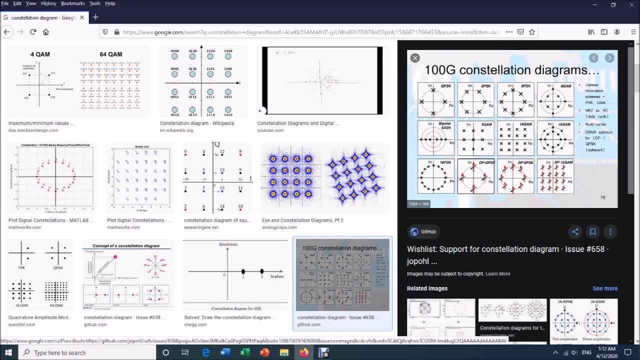 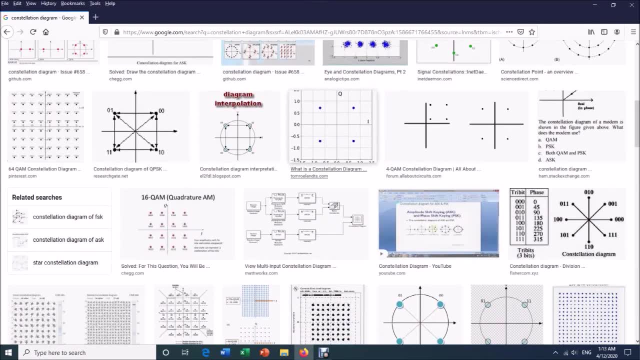 circumstances in designing the system. so and that's thankfully beyond the scope, and that's thankfully beyond the scope, and that's thankfully beyond the scope of our course. so feel free to look of our course. so feel free to look of our course, so feel free to look around. 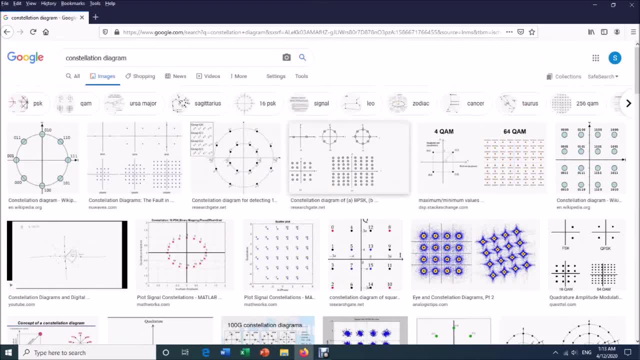 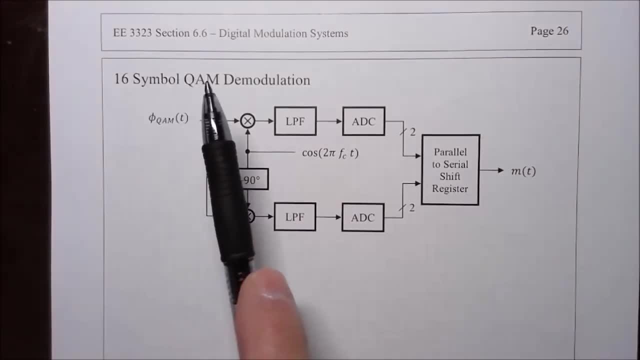 around around and see the various possibilities with, and see the various possibilities with, and see the various possibilities with constellation diagrams. they want to go constellation diagrams. they want to go constellation diagrams. they want to go through demodulation of the 16 symbol, through demodulation of the 16 symbol. 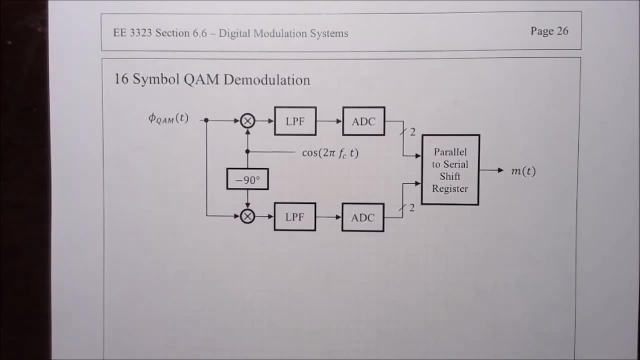 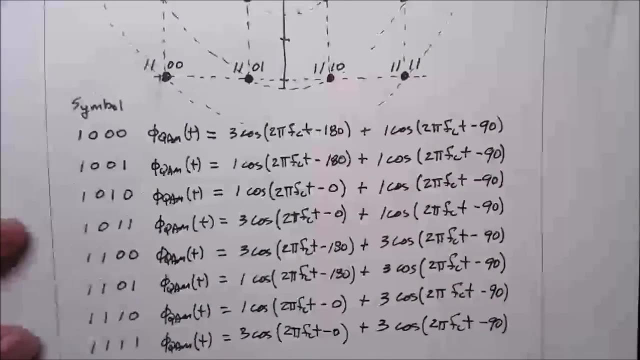 through demodulation of the 16 symbol: Q AM quadrature amplitude modulation. Q AM quadrature amplitude modulation. Q AM quadrature amplitude modulation- digital signal, but I'm certainly not digital signal, but I'm certainly not digital signal. but I'm certainly not going to do all 16, so I'm going to pick. 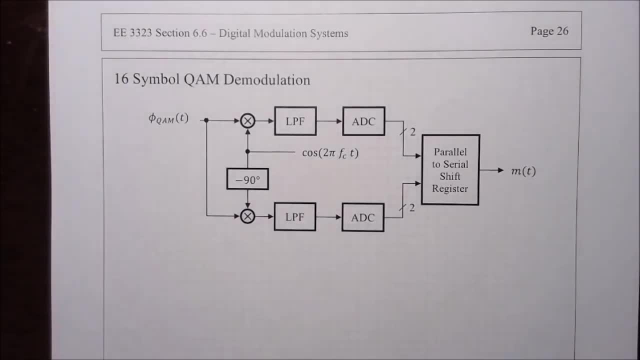 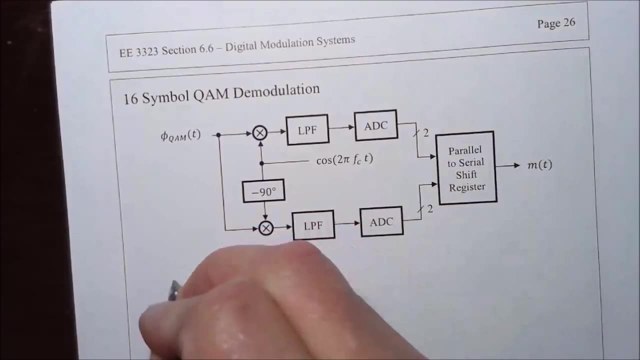 going to do all 16, so I'm going to pick, going to do all 16, so I'm going to pick one- maybe representative one, maybe representative one, maybe representative- and go through that demodulation and the and go through that demodulation and the. 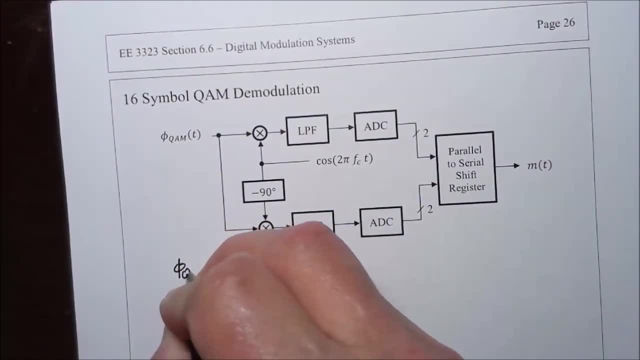 and go through that demodulation and the one I pick is: let's see which one do I. one I pick is: let's see which one do I. one I pick is: let's see which one do I pick. I don't want to tell you, so let's. 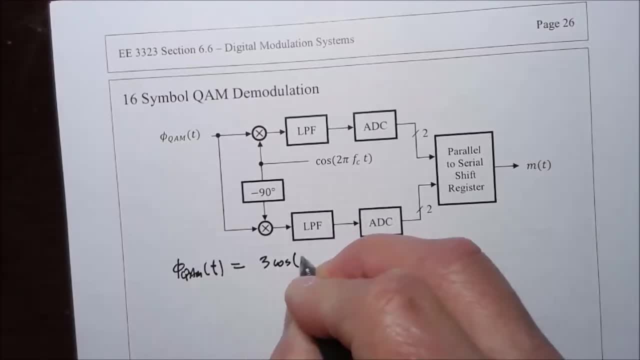 pick. I don't want to tell you, so let's pick. I don't want to tell you, so let's take a 3 times cosine 2 PI FCT minus 180. take a 3 times cosine 2 PI FCT minus 180. take a 3 times cosine 2 PI FCT minus 180 degrees. 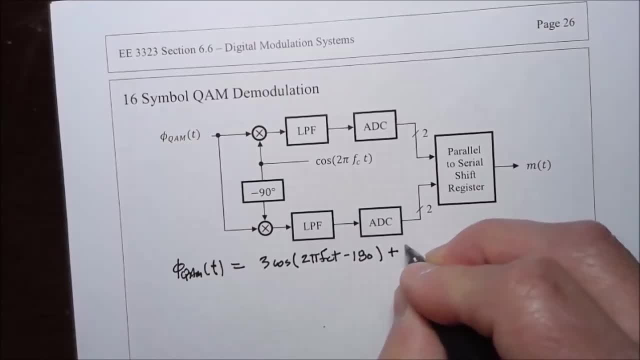 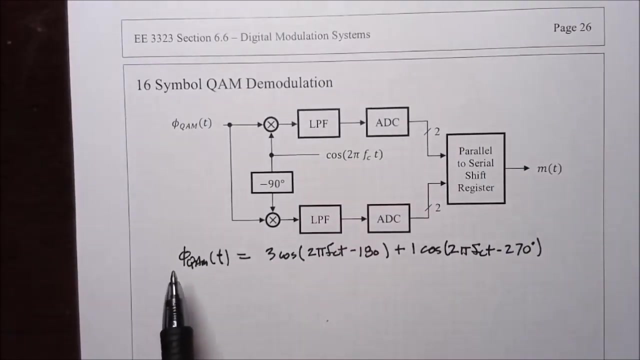 degrees: degrees plus plus plus one times cosine 2 PI FCT minus 270. one times cosine 2 PI FCT minus 270. one times cosine 2 PI FCT minus 270 degrees. okay, so this is this. this is the degrees. okay, so this is this. this is the. 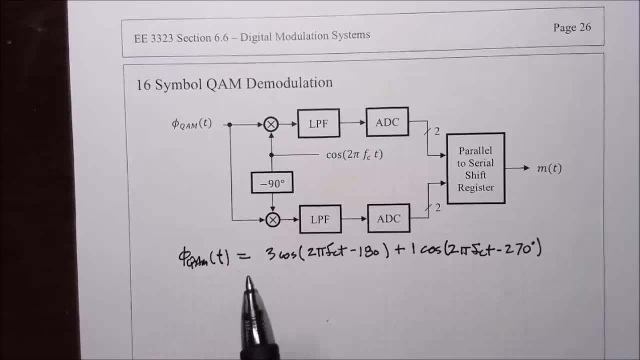 degrees. okay, so this is this, this is the quadrature AM signal for a particular quadrature AM signal, for a particular quadrature AM signal for a particular symbol, and I want to see what symbol symbol and I want to see what symbol symbol and I want to see what symbol that is by the process of this demon is. 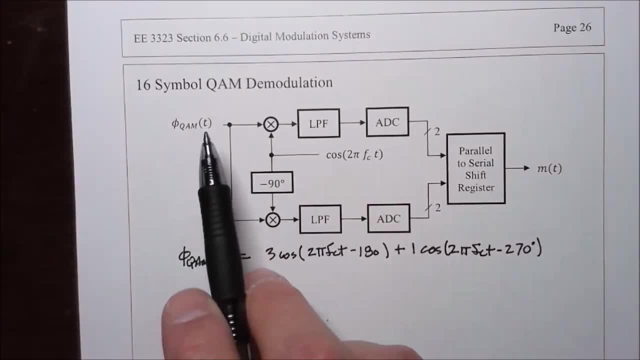 that is by the process of this demon, is that is by the process of this demon, is synchronous demodulation. so the signal synchronous demodulation, so the signal synchronous demodulation. so the signal is applied to a mixer and mixed with. is applied to a mixer and mixed with. 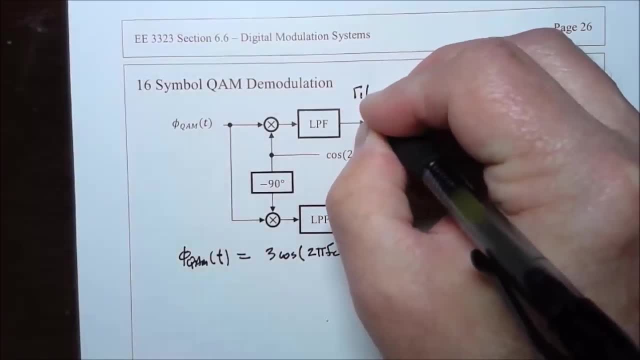 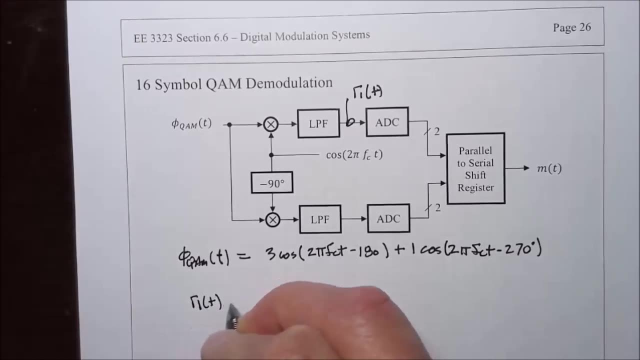 is applied to a mixer and mixed with this cosine pass to the low-pass filter. this cosine pass to the low-pass filter. this cosine pass to the low-pass filter. call this signal r1 of T. make r1 of T. call this signal r1 of T. make r1 of T. 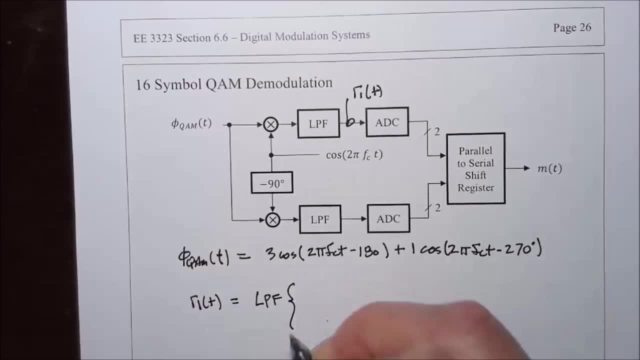 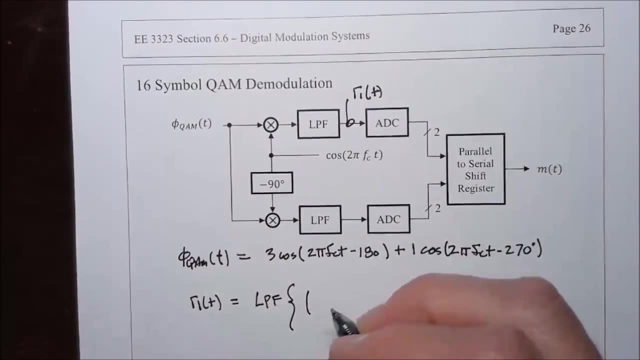 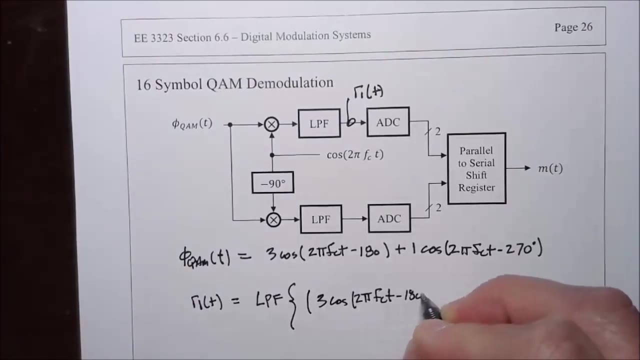 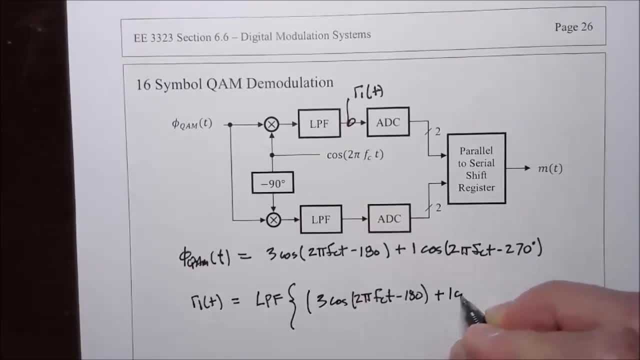 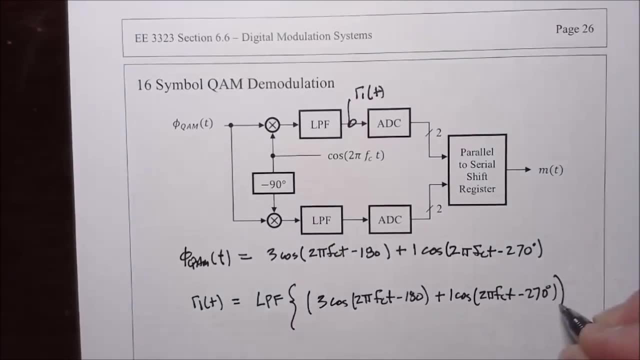 times the cosine 2 pi FCT minus 180 times the cosine 2 pi FCT minus 180 degrees, plus a 1 times cosine 2 pi FCT degrees, plus a 1 times cosine 2 pi FCT degrees, plus a 1 times cosine 2 pi FCT minus 270 degrees, we're going to 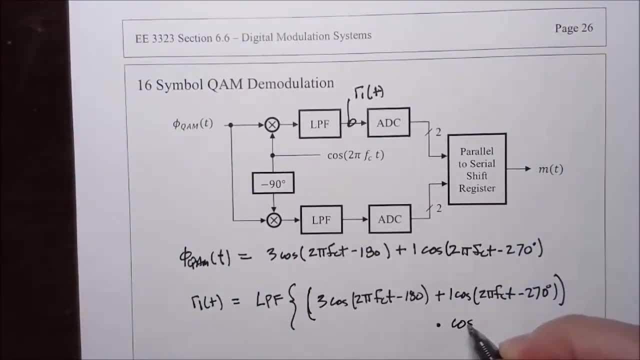 minus 270 degrees. we're going to minus 270 degrees. we're going to multiply that by cosine 2 pi FCT. okay, so multiply that by cosine 2 pi FCT. okay, so multiply that by cosine 2 pi FCT. okay, so this, this. 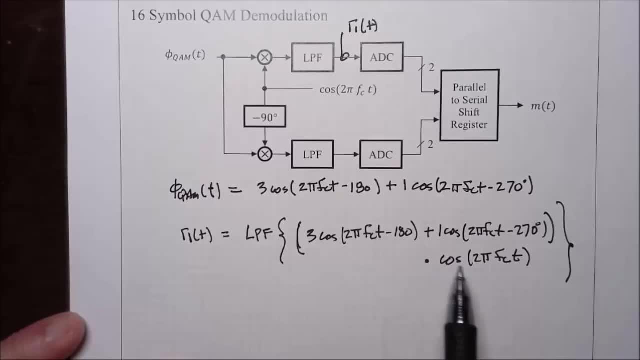 this sum it's some of these two cosines sum it's some of these two cosines. sum it's some of these two cosines. multiplies this cosine and we low-pass multiplies this cosine and we low-pass multiplies this cosine and we low-pass filter. that makes r1 of T equal to the. 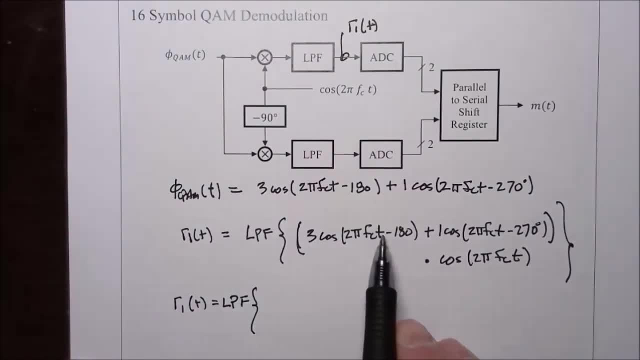 filter that makes r1 of T equal to the filter that makes r1 of T equal to the low-pass filtered version of cosine times. low-pass filtered version of cosine times. low-pass filtered version of cosine times cosine. let me apply the the trig cosine. let me apply the the trig. 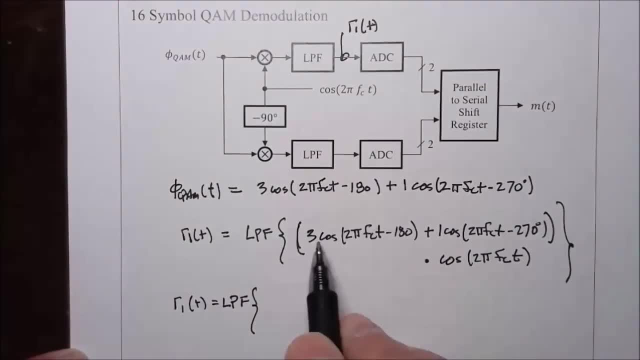 cosine. let me apply the the trig identity. we have 1 half times 3, 3 halves identity. we have 1 half times 3, 3 halves identity. we have 1 half times 3, 3 halves cosine of the difference between, cosine of the difference between. 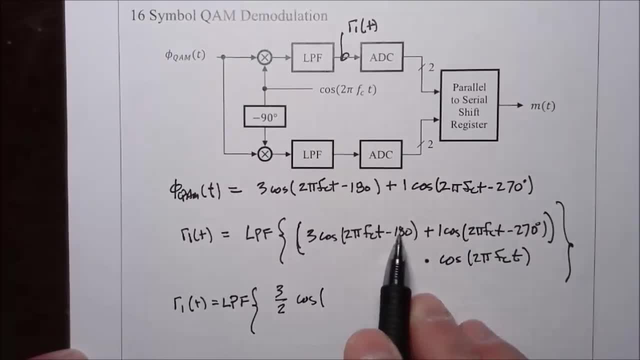 cosine of the difference between: of the two angles 2, 2 pi FCT minus 180. of the two angles 2, 2 pi FCT minus 180. of the two angles 2, 2 pi FCT minus 180 minus 2 pi FCT just leaves minus 180. 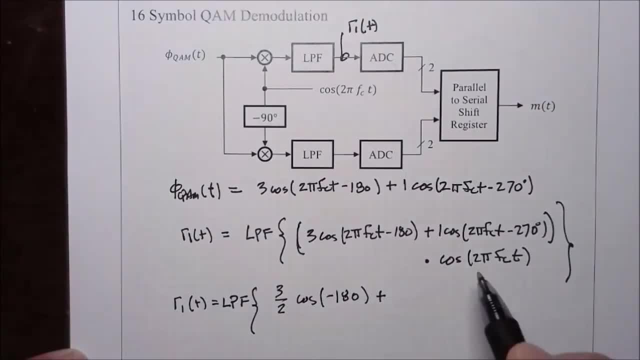 minus 2 pi FCT just leaves minus 180. minus 2 pi FCT just leaves minus 180. plus 3 halves cosine of the sum of the plus 3 halves cosine of the sum of the plus 3 halves cosine of the sum of the two angles: 2 pi times 2 FCT minus 180. 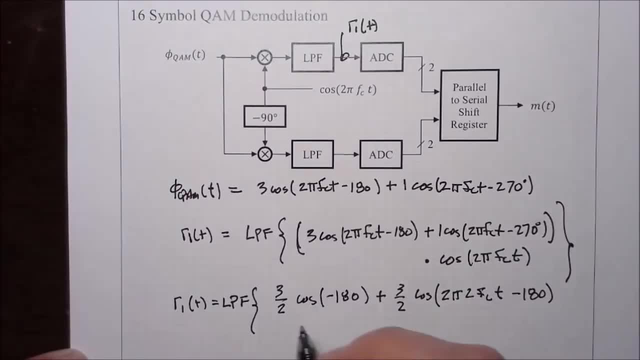 two angles, 2 pi times 2 FCT minus 180. two angles 2 pi times 2 FCT minus 180, and then the other multiplication gives, and then the other multiplication gives, and then the other multiplication gives us, us, us plus 1 half cosine, the difference of the. 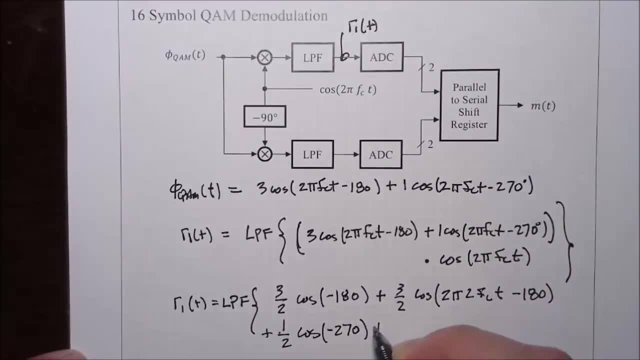 plus 1 half cosine, the difference of the plus 1 half cosine, the difference of the angles, and it's 270 degrees plus 1 half angles, and it's 270 degrees plus 1 half angles and it's 270 degrees plus 1 half cosine, 2 pi times 2 FCT minus 270. so 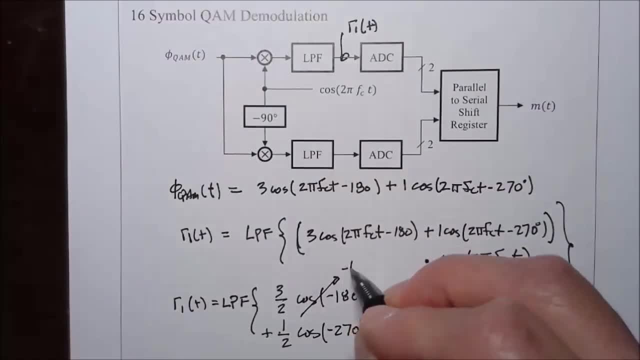 cosine 2 pi times 2 FCT minus 270, so cosine 2 pi times 2 FCT. minus 270, so cosine minus 180 it's minus 1 cosine, and cosine minus 180 it's minus 1 cosine, and cosine minus 180 it's minus 1 cosine and minus 270 is 0. low-pass filter takes out. 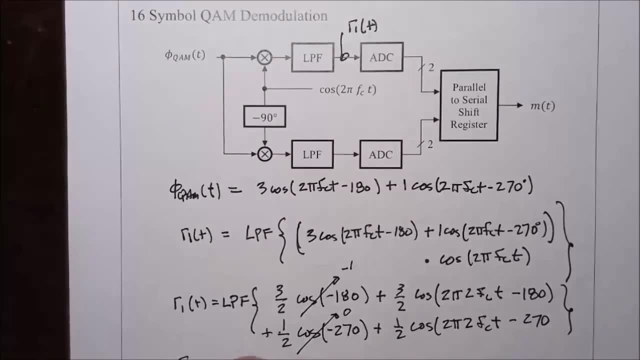 minus 270 is 0. low-pass filter takes out: minus 270 is 0. low-pass filter takes out the two high frequency components, the two high frequency components, the two high frequency components. then R 1 of T is going to be equal to. then R 1 of T is going to be equal to. 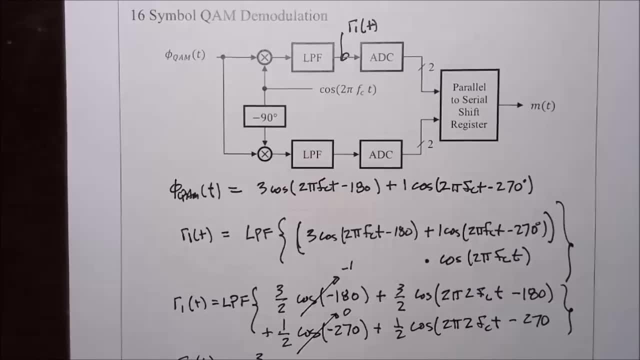 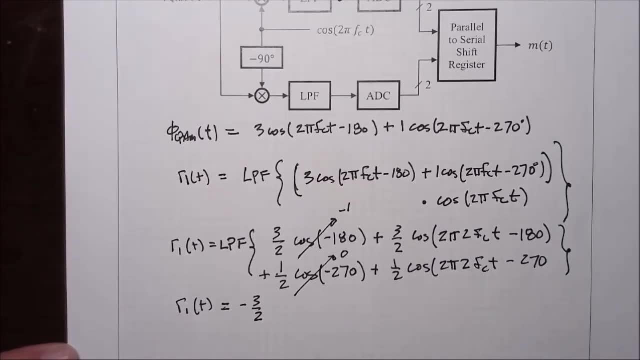 then R 1 of T is going to be equal to minus 1 times 3 halves, minus 3 halves, minus 1 times 3 halves, minus 3 halves, minus 1 times 3 halves, minus 3 halves, minus 3 halves, which we've got, we've got. 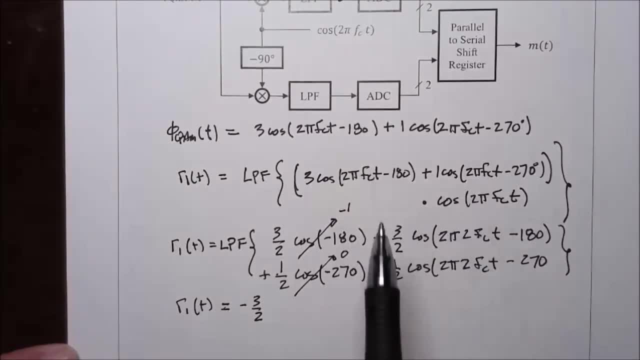 minus 3 halves, which we've got. we've got minus 3 halves, which we've got. we've got the thing scaled by 1 half because of the thing scaled by 1 half, because of the thing scaled by 1 half because of the the trig identity. but we could easily. 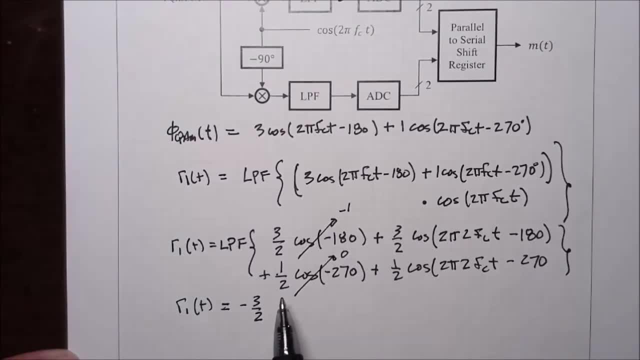 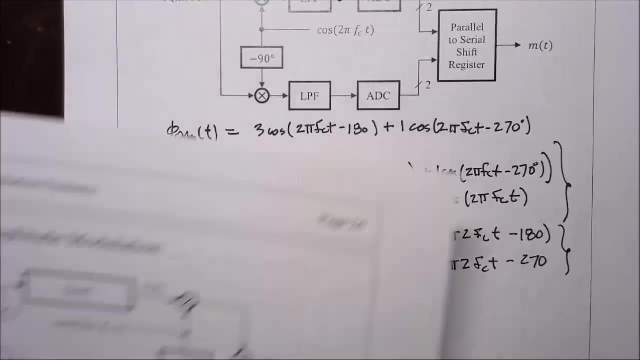 the the trig identity. but we could easily the the trig identity, but we could easily, we would, could easily amplify the, we would, could easily amplify the, we would, could easily amplify the. this by a factor of 2 and this minus 3 on our. this by a factor of 2 and this minus 3 on our. 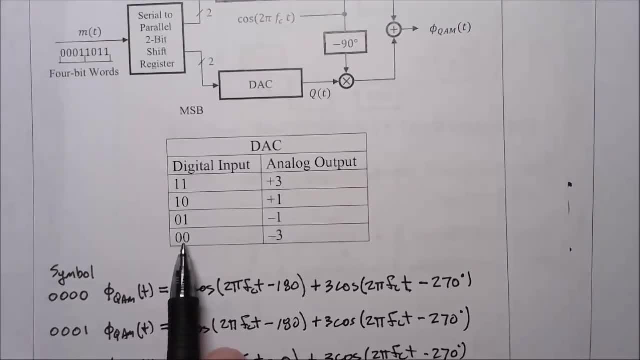 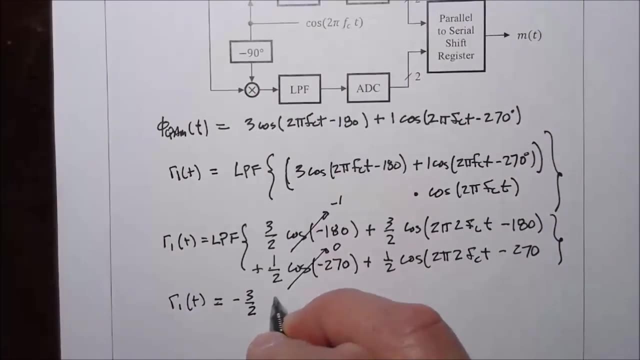 this by a factor of 2 and this minus 3 on our on our chart maps to a: 0: 0 is the. on our chart maps to a 0: 0 is the on our chart maps to a 0: 0 is the least significant bits, so this maps to the. 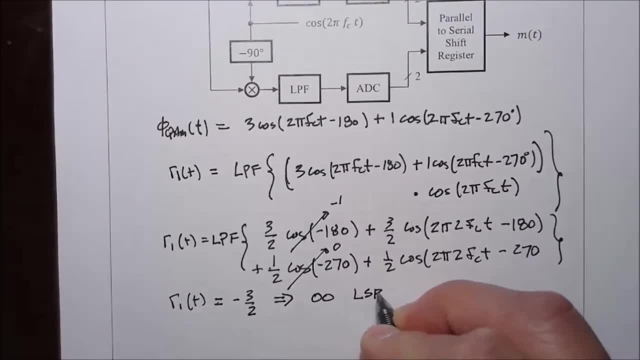 least significant bits. so this maps to the least significant bits. so this maps to the symbol 0, 0 for the least significant symbol. 0, 0 for the least significant symbol: 0, 0 for the least significant bits. then if we, if we turn bits, then if we, if we turn, 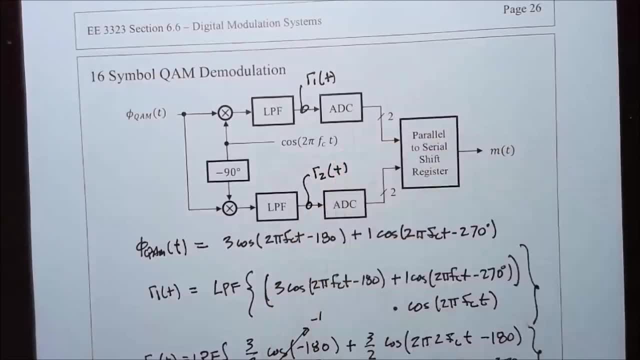 bits. then if we, if we, if we turn around and find our 2 of T that's equal to the around, and find our 2 of T that's equal to the around, and find our 2 of T that's equal to the low-pass filtered version of again. 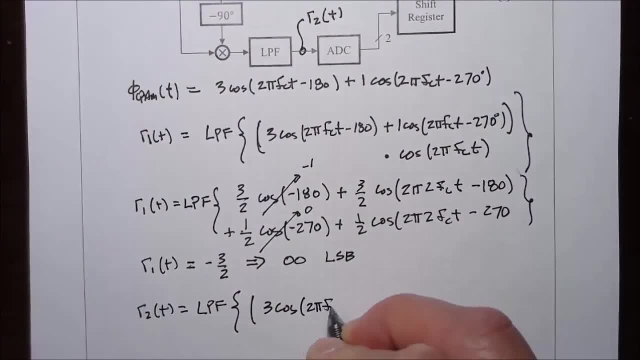 low-pass filtered version of again low-pass filtered version of again: 3 cosine 2 PI FC T minus 180 degrees plus 3: cosine 2 PI FC T minus 180 degrees plus 3: cosine 2 PI FC T minus 180 degrees plus 1 cosine 2 PI FC T minus 270 degrees. 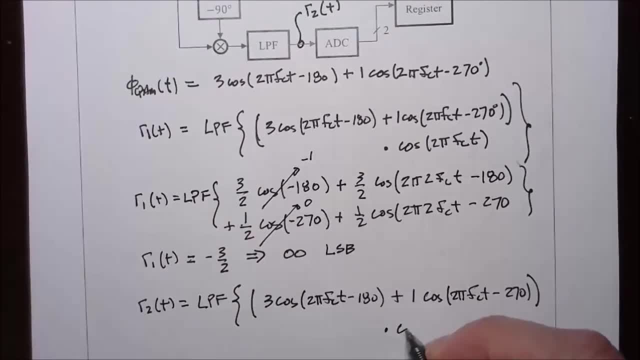 1 cosine 2 PI FC T minus 270 degrees, 1 cosine 2 PI FC T minus 270 degrees, and that all multiplies cosine 2 PI FC T, and that all multiplies cosine 2 PI FC T, and that all multiplies cosine 2 PI FC T minus 90 degrees. here we're multiplying. 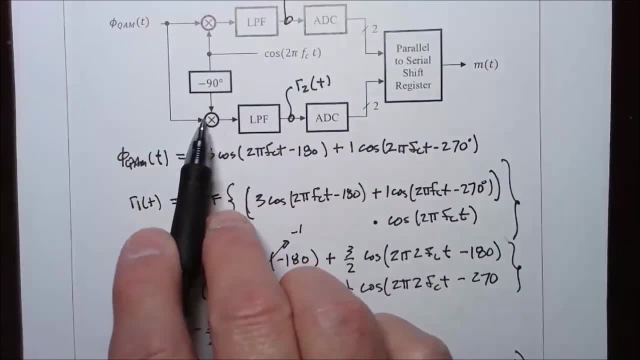 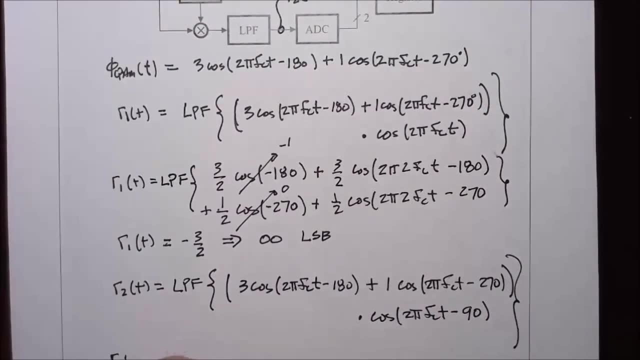 minus 90 degrees. here we're multiplying minus 90 degrees. here we're multiplying by the phase, by the phase, shifted by the phase, by the phase, shifted by the phase, by the phase shifted. version of the carrier. and that makes version of the carrier and that makes 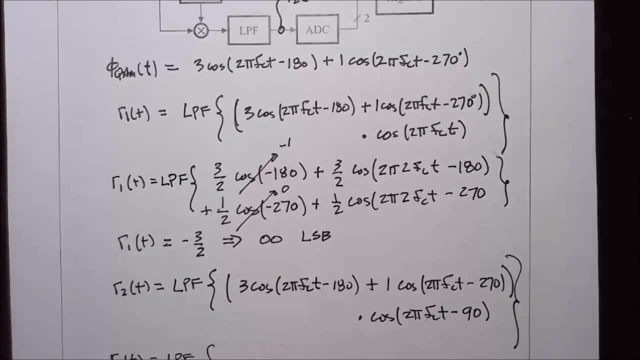 version of the carrier and that makes the signal the low-pass filtered version, the signal the low-pass filtered version, the signal the low-pass filtered version of C. we have cosine times a cosine it of C. we have cosine times a cosine it of C. we have cosine times a cosine it just gives us 3 1⁄2 cosine of the. 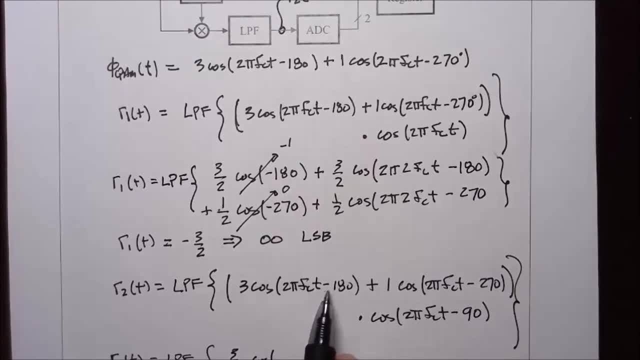 just gives us 3 1⁄2 cosine of the just gives us 3 1⁄2 cosine of the difference of the angles, which is going difference of the angles which is going difference of the angles which is going to be minus 180, minus a negative 9. 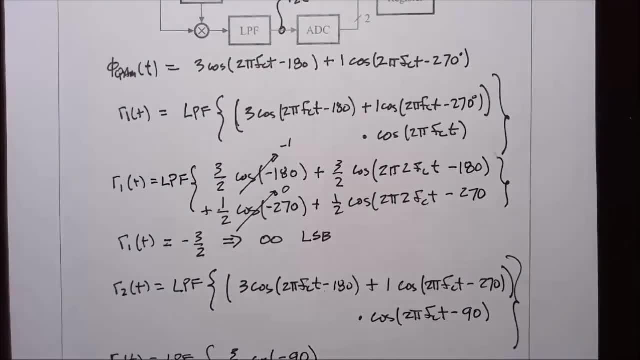 to be minus 190, so that ends up to be to be minus 190, so that ends up to be to be minus 190, so that ends up to be minus 90 degrees plus 1, 3 halves. I'm. minus 90 degrees plus 1, 3 halves I'm. 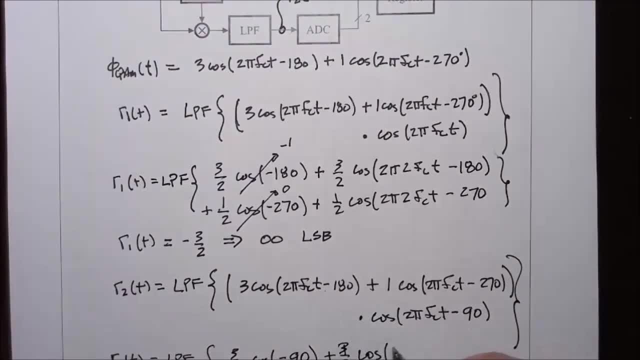 minus 90 degrees, plus 1, 3 halves- I'm sorry- 3 halves cosine of the sum of the sorry. 3 halves cosine of the sum of the sorry. 3 halves cosine of the sum of the angles: 2 PI times 2 FC T minus 270. 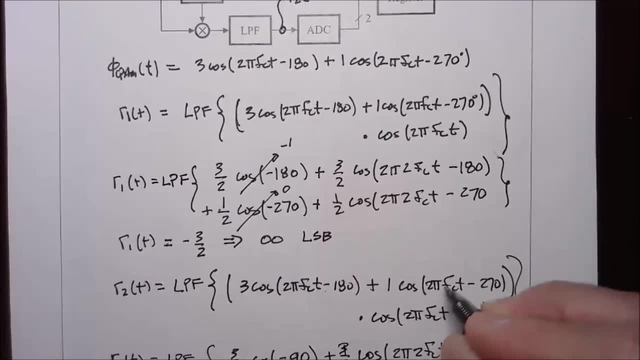 angles: 2 PI times 2 FC T minus 270 angles: 2 PI times 2 FC T minus 270. degrees plus for the other cosine times. degrees plus for the other cosine times. degrees plus for the other cosine times: a cosine is 1 half cosine the difference. 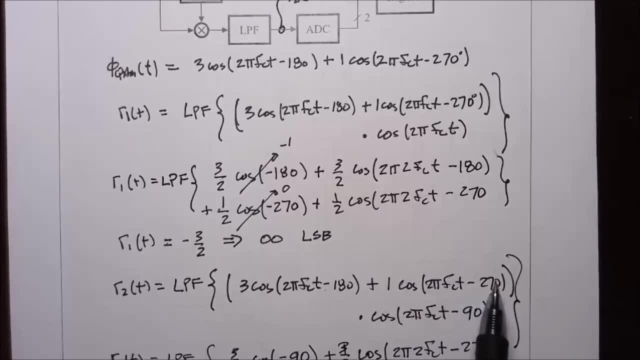 a cosine is 1 half cosine. the difference- a cosine is 1 half cosine. the difference of the angles minus 270, of the angles minus 270 of the angles minus 270 plus 90, would you give us minus 180 plus 90, would you give us minus 180. 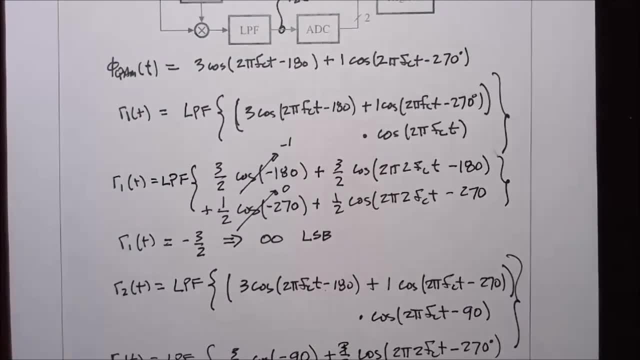 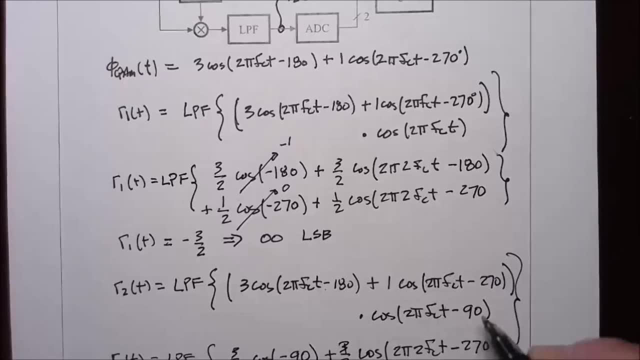 plus 90, would you give us minus 180 degrees, plus 1 half cosine of the sum degrees, plus 1 half cosine of the sum degrees, plus 1 half cosine of the sum, and that's going to be looks like minus and that's going to be looks like minus. 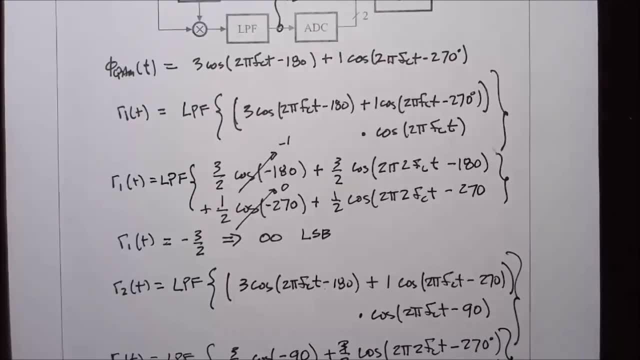 and that's going to be looks like minus 360 degrees. the cosine of minus 90 is 360 degrees. the cosine of minus 90 is 360 degrees. the cosine of minus 90 is 0. cosine of minus 180 is minus 1: 0. cosine of minus 180 is minus 1.